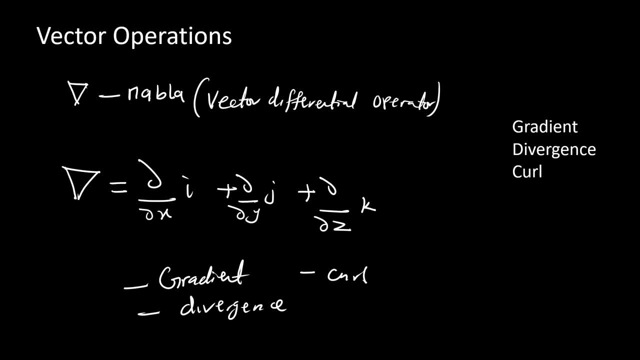 So, using this operator, we can determine our gradients, our divergence and our curl. So, taking the data from this value, we are going to be using NABLA in this tutorial And know that NABLA is defined as the partial derivative of X in direction of I, plus the partial derivative of Y in direction of J, plus the partial derivative of Z in direction of Z. 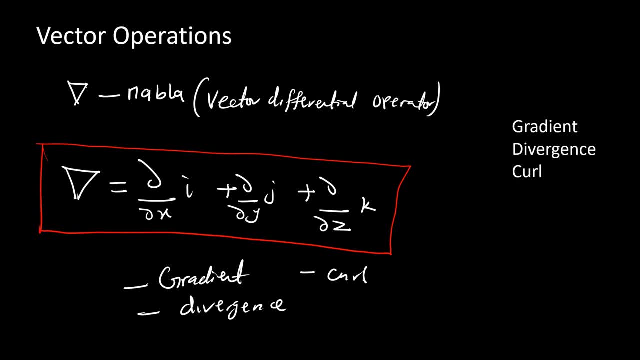 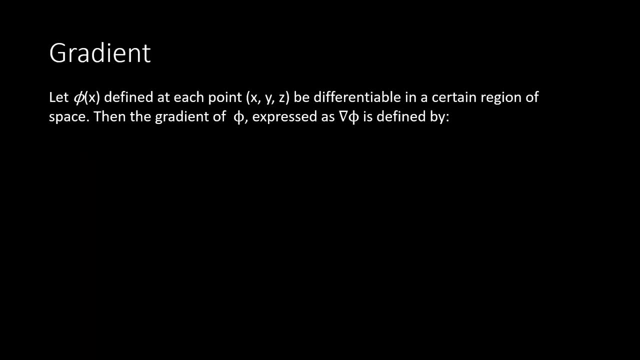 z in direction of k. so let's get started with the meaning of gradient divergence and call to start. we are going to be looking at gradient gradient, so let phi define at each point x, y and z, taking that phi is a function of x defined at each point x, y and z to be differentiable. 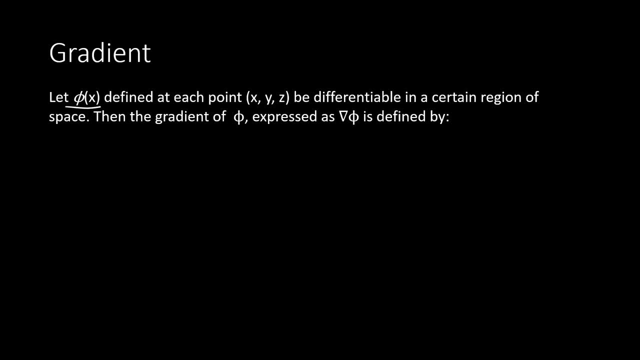 in a certain region of space, then the gradient of phi expresses nabla. phi is defined as so wherever you see something like nabla and the function, this is also as gradient. when we reach divergence, we also talk about how we can denote our divergence, but in this case we denote gradient as. 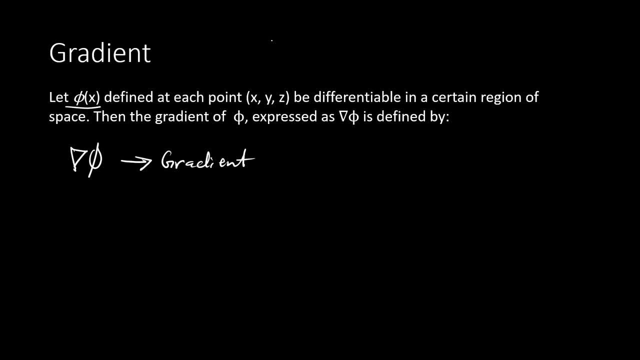 phi as nabla phi. as we are looking for the degree of a function with vector f, the gradient of f is going to be nabla f. hope you get it. if you're looking for the gradient of a function or effect of value function, which is a, then the gradient of a is going to be nabla a. so this dimension is simply the gradient of. 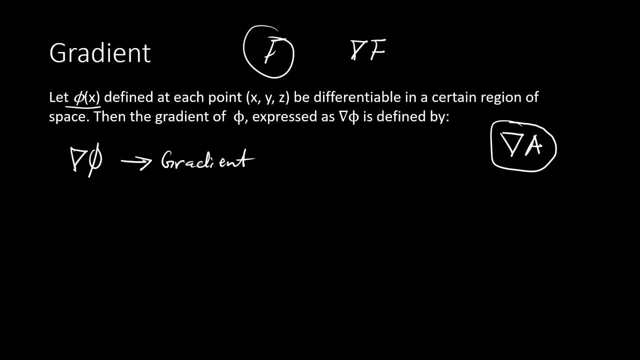 a. now we define our nabla a. don't forget, in the previous slide we look at nabla to be equal to the partial derivative of x in direction of i, plus the partial derivative of y in the direction of j, plus the partial derivative of z in direction of k. so in this case of gradients we're going to have: 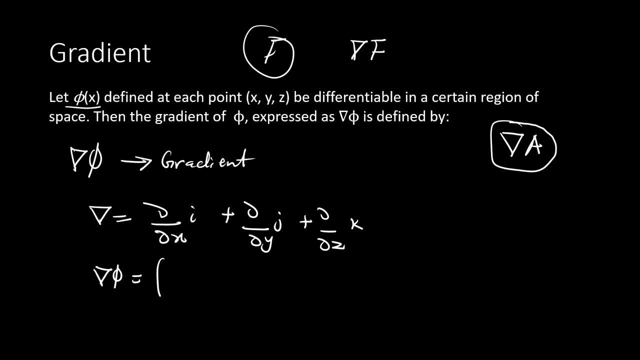 our nabla phi to be equal to nabla, multiply by phi. so here we have the partial derivative of x in direction of i, plus the partial derivative of y in direction of j, plus the partial derivative of z in direction of k. then multiply by phi, so then you can choose to open this bracket. 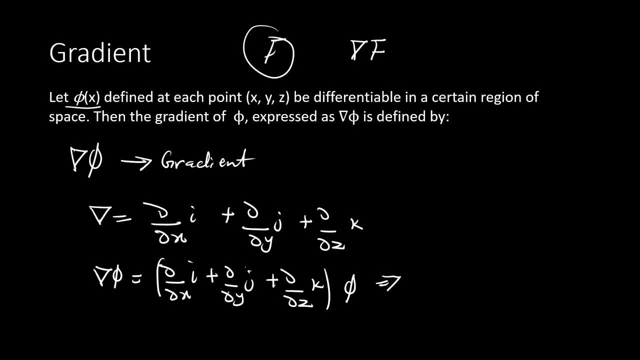 so in this case we are going to have that, our nabla phi, equal to the partial derivative of phi in direction of i, plus the partial derivative of phi in direction of j, plus the partial derivative of phi in direction of k. so take note of this very way. this is simply the representation of 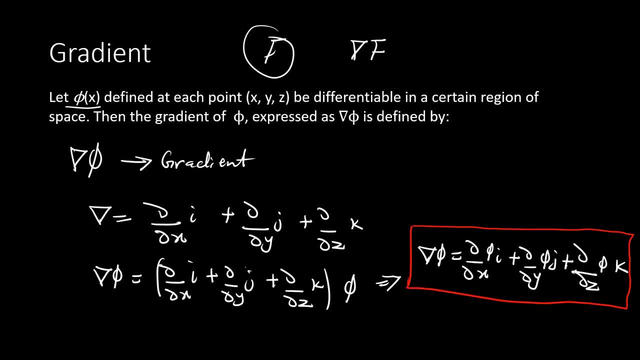 gradient. so take note, you have certain from a. you know that phi, nabla. phi is our gradient. so we have our nabla already defined as the partial derivative of x9 of i, plus the partial derivative of y in direction of j, plus the partial derivative of z in direction. 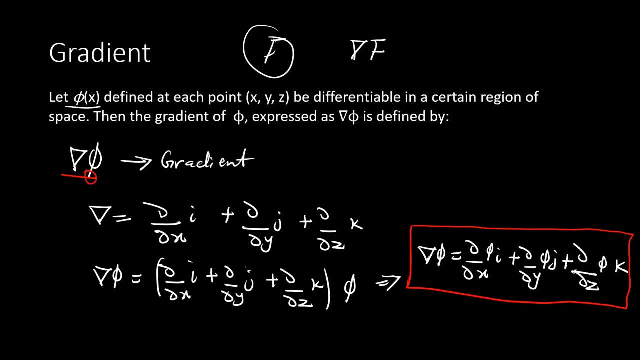 of k. so we are simply multiplying our function, which is phi, by nabla. so this is what we have in this case: this is our nabla and this is phi. so we are multiplying our phi by our nabla, so opening these brackets. so phi is going to be distributed to three terms: this term, this term. 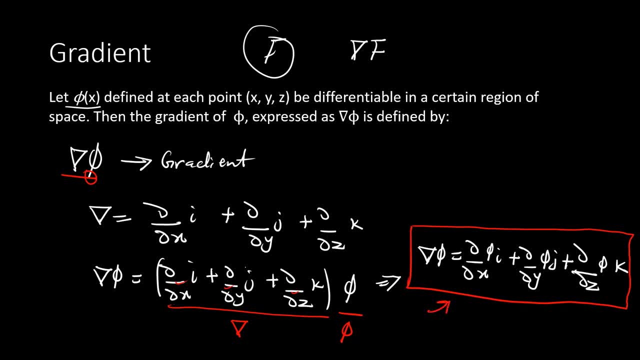 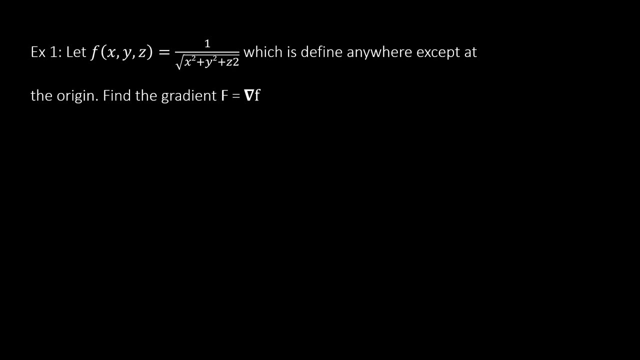 and this term, and that's what leads us to this. so this is our representation of gradient. if i have to find gradient, we simply take the partial derivative of the function in relation to x, y and z. let's look at an example. this is first example we are going to be looking at. the equation states: 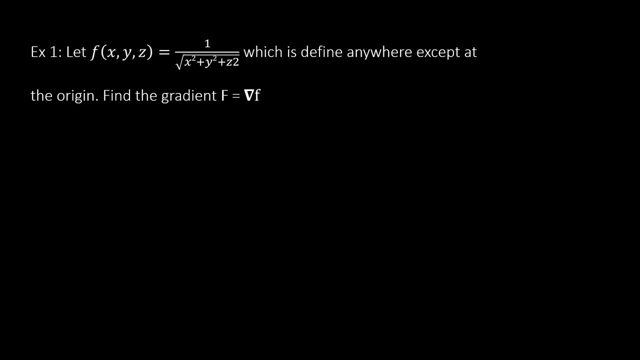 let f of x, y, z, equal to one over the square root of x square plus y square- i'm sorry, supposed to be z square- which is defined anyway, except at the origin- find the gradient f. so in this question we have to find the gradient of f, which is nabla f. so our function is f and the gradient of f is. 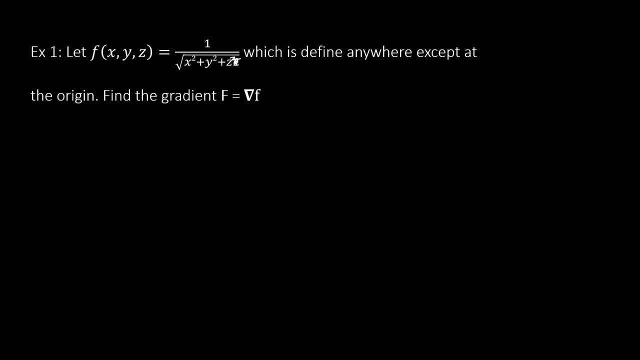 going to be nabla f. so let's write out our function. f is a function of x, y and z equal to 1 over the square root of x square dot, the square root of y square, plus the, the square root of z squared. so this, our function, is defined, which is function. 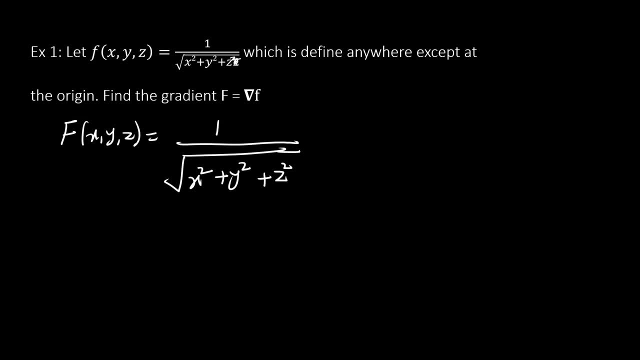 f. so we have to look for nabla f, which is the gradient of f. so our nabla f is going to be: so let's write out our expression for nabla d over dx. direction of i plus d over dy. direction of j plus d over dz, direction of k. 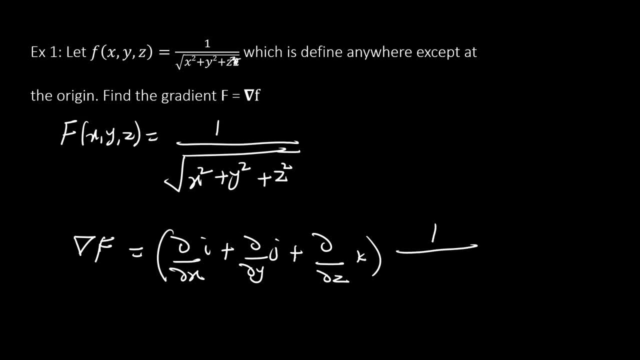 so we put our f, which is 1, over the square root of x squared plus y squared plus z squared. so this is what we have: first the f, which is our nabla, f, which is the gradient of f equal to nabla. this is nabla, just take note of this very way. and this is f. so now we multiply through by f. 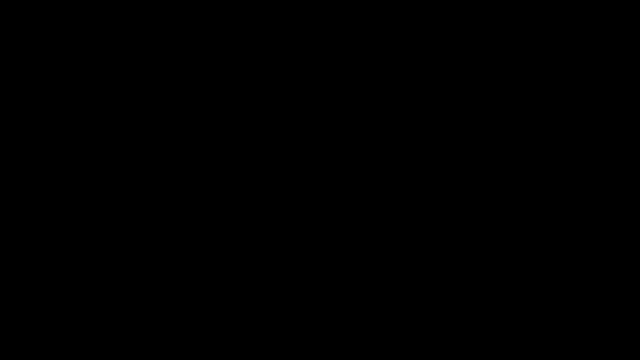 so in this case we are going to have our nabla f to be equal to the partial derivative of of 1 over the square root of x squared plus y squared, plus z squared in direction of i, plus the partial derivative of 1 over the square root of x squared plus y squared plus z squared. 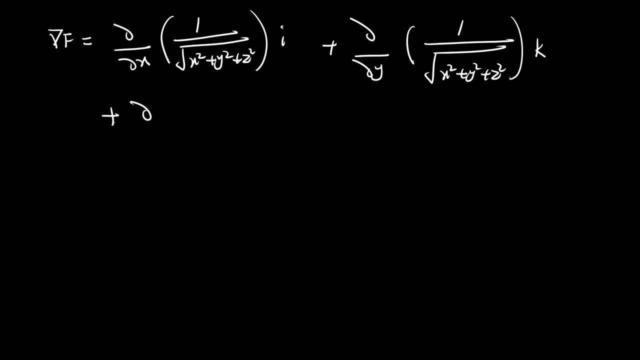 in direction of k, plus the partial derivative of 1 over the square root of x squared plus y squared plus z squared in direction of k. so we have to look for this, this and this, so the addition of this still is going to be our answer, which is the gradient of f, nabla, f. so let's take this one after the other. 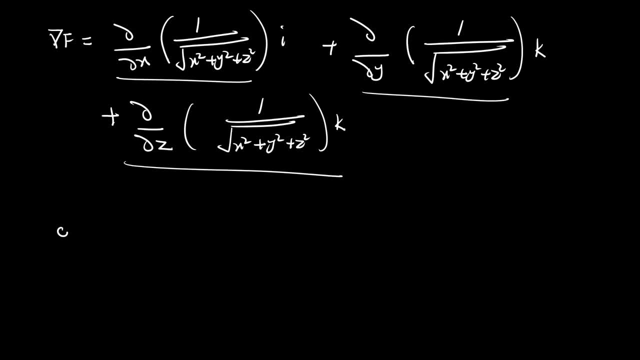 the first one is the partial derivative of. so we differentiate with respect to x. so what we know about and what we want, if we are going to differentiate with respect to x, will be właśnie our function, f, nabla, f, ii, because ii is now part of one and a half. 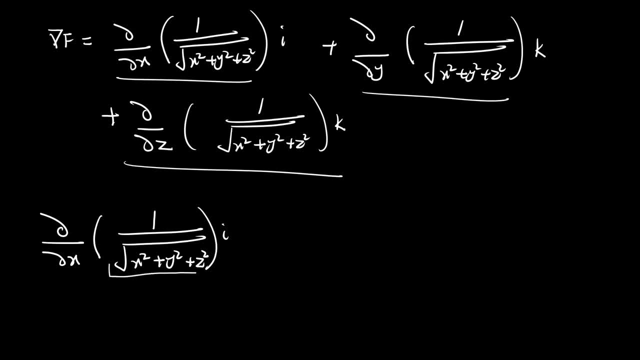 so the difference to do is to differentiate this term with respect to x. so the first time to do is to differentiate this term with respect to x. and if you are differentiating with respect to x, we are going to treat y and z as constant. so i'm going to treat this as normal integral. let me 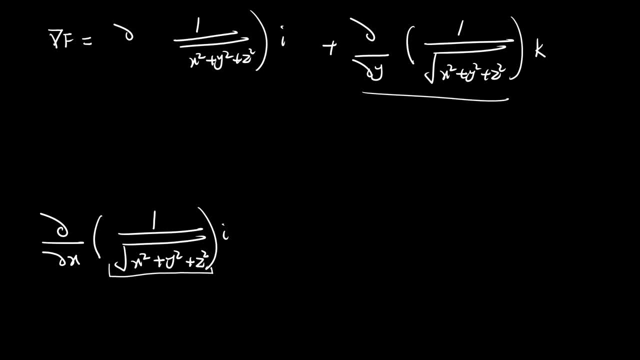 clean this off. so we treat these ones as normal integral. so we talk about this only as just an, as just an entity, without looking at the partial derivative for looking at it as a factor valued function. so let's try to differentiate, with respect to x, this function, one over the square root of a square plus y square plus z square. so let's try. 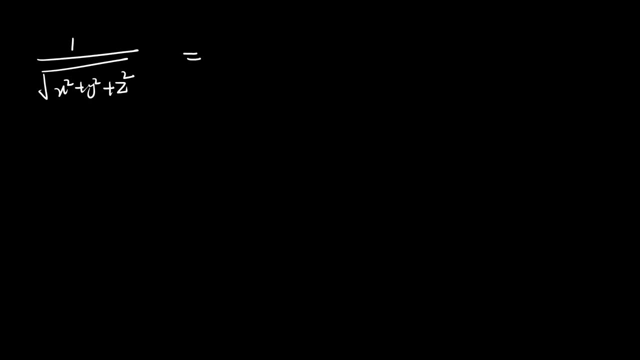 to differentiate this function with respect to x, so we can simplify this further to be equal to one over x square plus y square plus z square. this is one over two. so if we remove one over, we can change this into f square plus y square plus z square to the power of minus one over two. 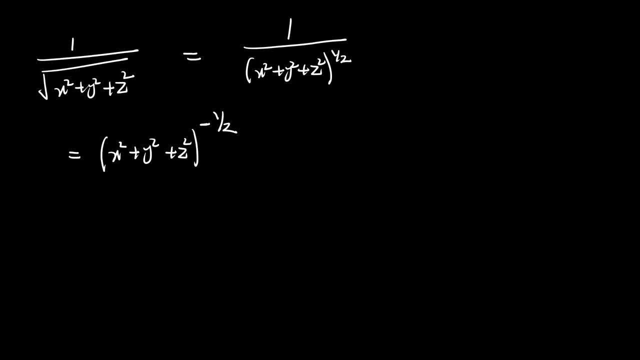 so i've removed one over there. so to differentiate on nomaday with respect to x, let's set our u- this is going to be a function of a function- our u to be equal to x square plus y square plus z square, and therefore the u over the x, since we are 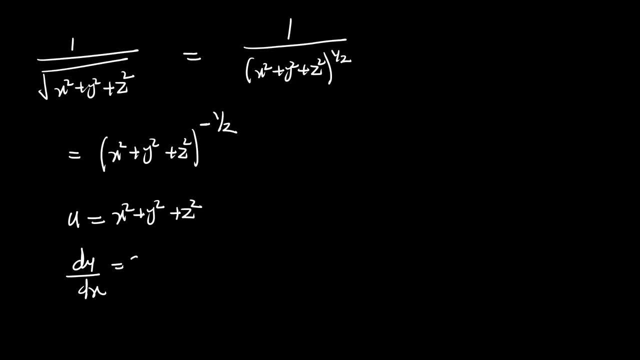 differentiating with respect to x. the u for this is going to be 2x. and don't forget, we are differentiating with respect to x. we are treating y and z as constants, so that's our du. for the x, so we get, our y is going to be u to the power of minus 1 over 2, right, so our dy over du. 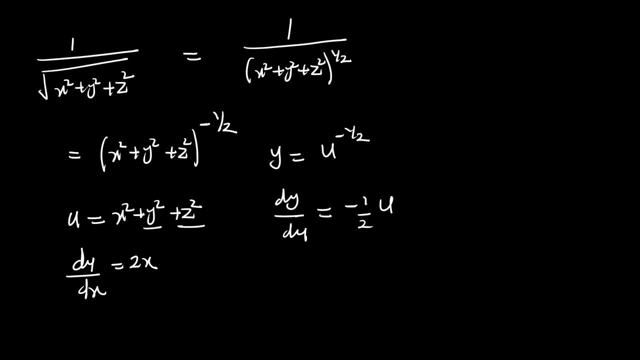 equal to minus 1 over 2, u minus 1 over 2 minus 1, and then we are going to have minus 1 over 2, u minus 3 over 2, minus 1 over 2, u minus 3 over 2. so we can also simplify this further. 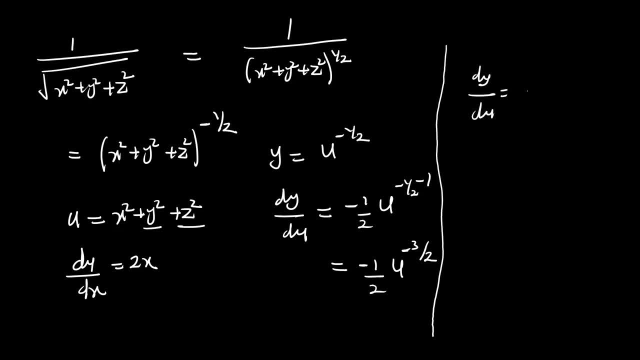 let's say our dy over du, equal to minus you minus 3 for 2 over 2. so don't forget, we are trying to treat this entity as just an independent variable. so we have forget our dy over dx. now we are forgetting our respect to x or respect to y, we are forgetting. 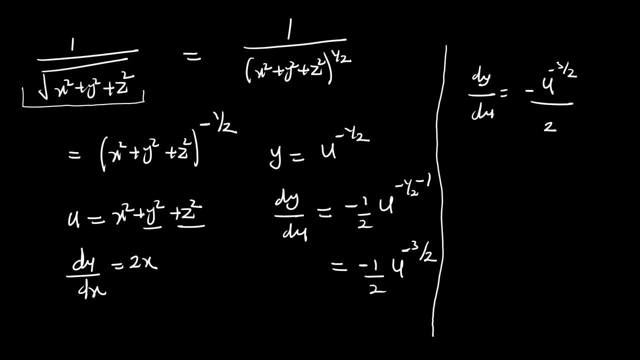 that we are looking at a factor function. we want to treat this as a normal differentiation. so we have our du over du to be this, and we have our du over dx to be this. so let's use the formula for function of a function to derive the answer now. 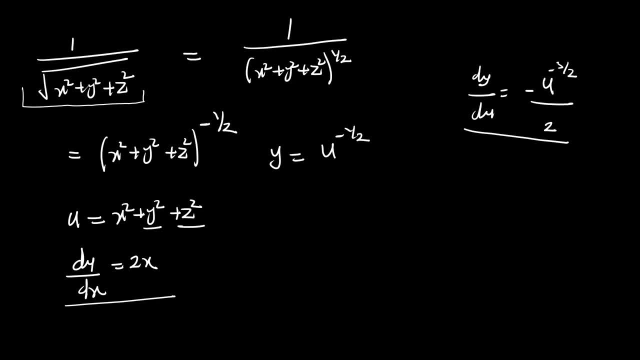 we're going to have our dy over dx. so the y is equal to the y over the y that the x. so we are going to have our dy over the x to be equal to the y over the u, times du over dx. so our dy over the u is: 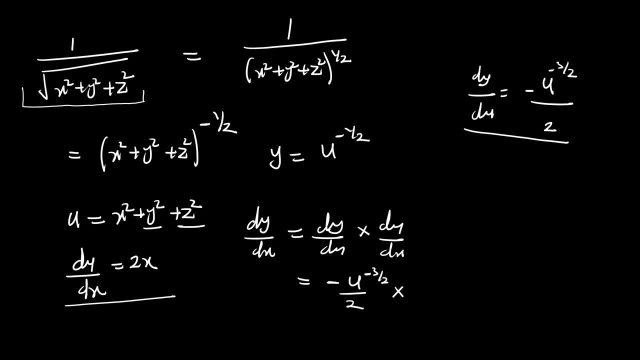 minus u over 2 to the power of minus 3 over 2 times our du over dx, which is 2x. so yeah, to cancel out. I have this because minus X you minus 3 over 2, minus X you minus 3 for 2. so I'm going to working with this, as I mentioned. 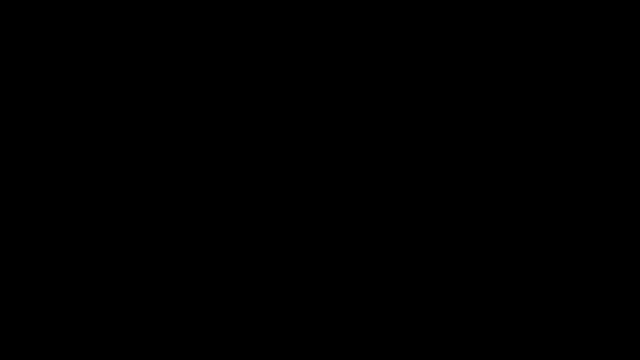 earlier. so I do. I for DX is minus X, you minus 3 for 2, so let's try to substitute all our values for you. so we have this to be got minus X or play-by-ways s, K plus Y square plus Z square to the power. 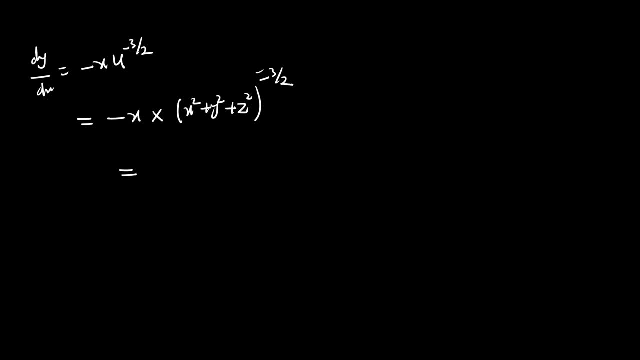 this manor, but I mean this: you, you, you minus X. apply by 1 over x square plus y square plus Z square, to the power of 3 for 2. so I'm just doing this to remove this negative sign. so this is going to be 1 over and if you simplify this further, we are going to have this to be: 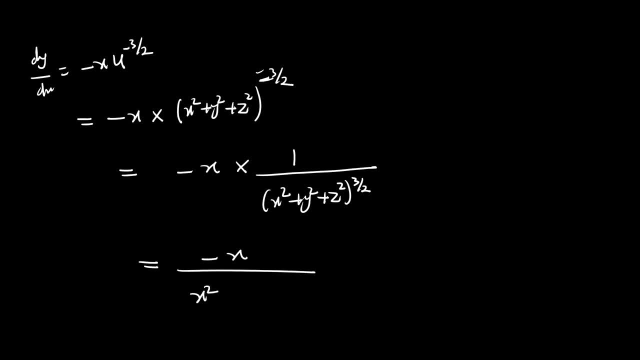 equal to minus X over x square plus y square plus Z square. so it is simply about partial derivative with respect to X of F. I hope you understand that. so this is simply about partial derivative with respect to X. if you differentiate F with respect to x, this is what you are going to have. note, where this shows that you are differentiating with respect. 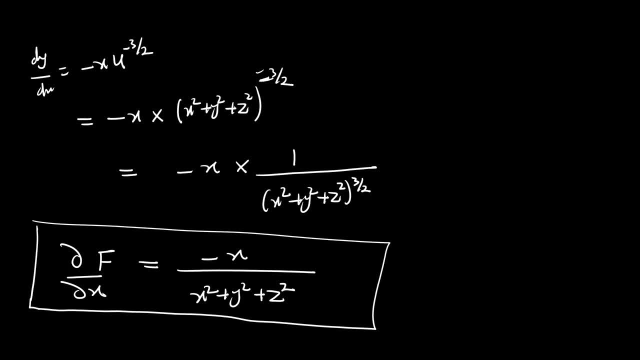 to X is that we are treating y and Z as constant and we differentiated X. so therefore we have minus X over x square, plus y square, plus Z square. so similarly over the y is going to be- you can try this out- but it's going to be minus y over. 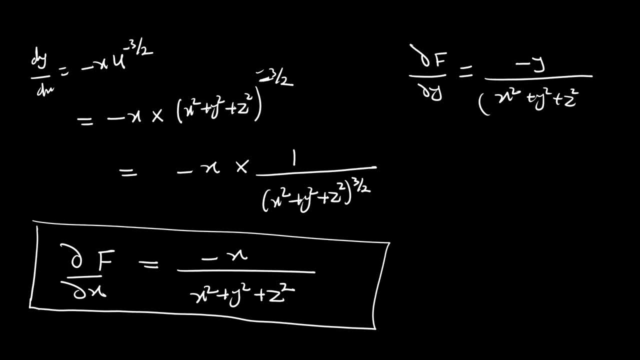 s squared plus y squared plus z squared. well, three over two, and also, if i differentiate with respect to z is going to be minus z over a square, plus y squared plus z squared. so these are the three values that we are going to be making use of. 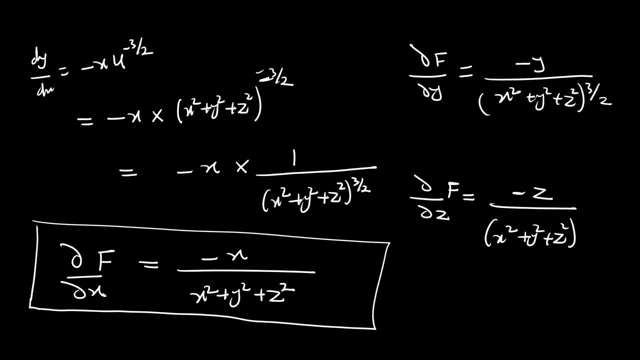 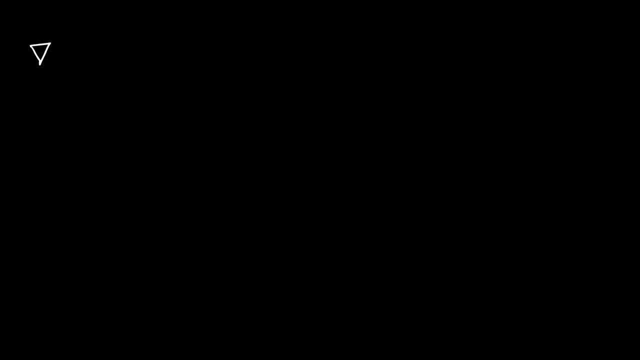 in writing the answer to this question. so let's write the answer now. this will be now of our unit of f, which is the number f to be caused by your derivative with respect to f which is related to x, i plus partial derivative with respect to y. 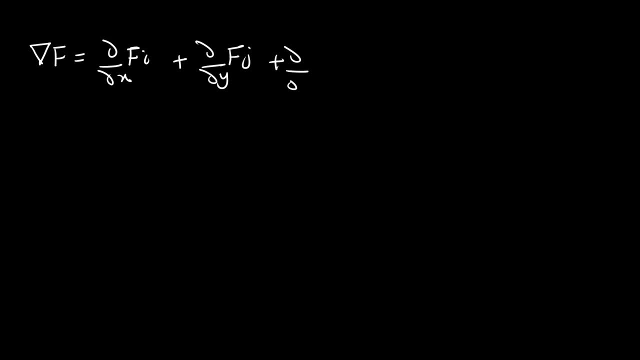 j, plus partial derivative with respect to z in direction of k. so let's write this out one after the other, so you have this first time to be equal to minus x over x squared, plus y squared plus z squared. if there's nothing, there's anything you don't understand, feel free to post. 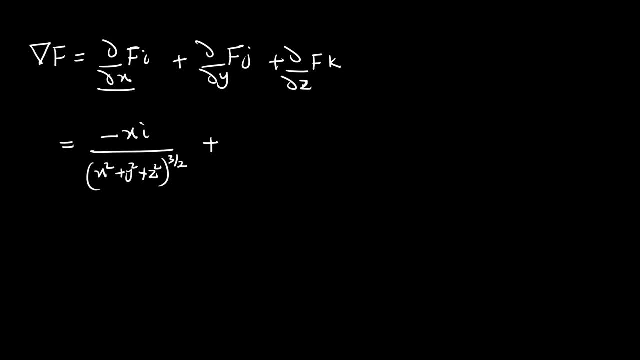 your answer in your question in the comment section below: and this time is going to be minus y j over s squared plus y square plus z, squared three for two plus, and this time is going to be minus z k over s squared plus y squared plus z. 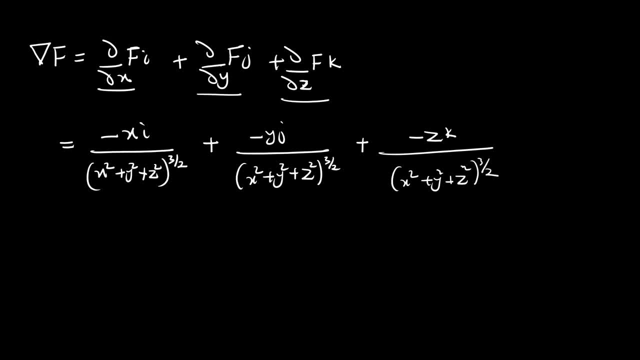 squared three for two, and since we have common denominators, this can also be written as minus x и plus y, j plus z k. so now i'm factorizing out negative through this center of our denominator, which is x square plus y square plus z square, to the power of 3 for two. and 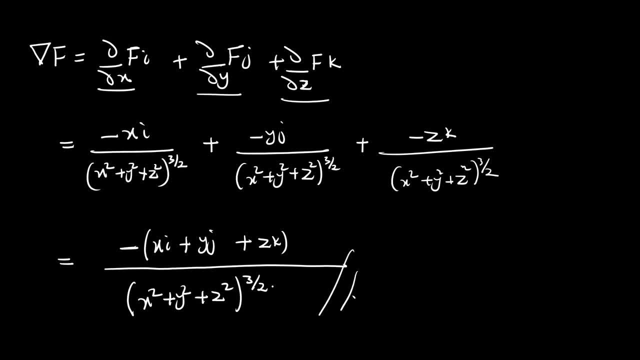 this is the answer to our question, which is the gradient of f. when this is the gradient of f, you can simplify this further by looking at a circle, by converting this to be like equation of a circle. but there's not much need for that, so we are going to stop our answer. a. so if you have to convert, 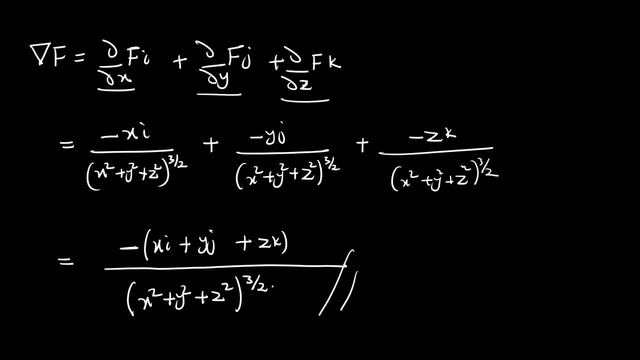 this to equation of the circle. let's go to that. if i convert this to equation of circle, we can treat all of this to be equal to r. so we are going to have minus r over. then you can treat all of this, since this is simply equal to the cube root of all this function, square. so this is going to be. 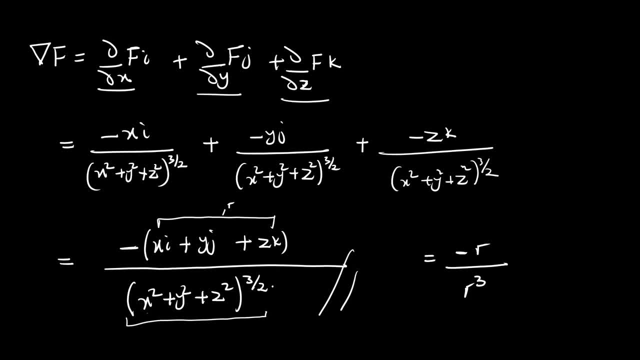 r cube, since this is simply the square root of all this function, to the power of three. so this is going to be minus r over r cube. so that is, if you have to treat this as an equation of a circle. so this, simply, i will derive our answer, which is nabla f, which is the gradient of f, we. 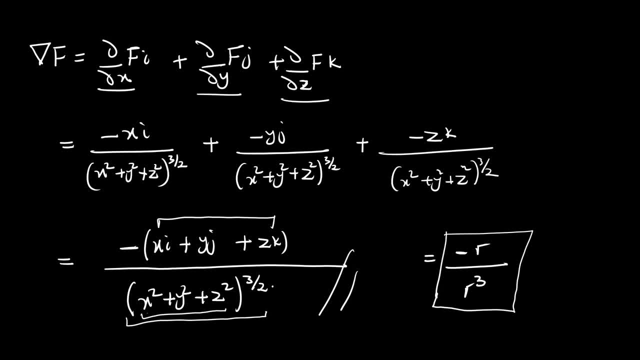 look at: we differentiate f with respect to x, we differentiate f with respect to y by keeping the other, the other variables, constant, and we differentiate with respect to z by keeping the other variables constant, and we write them out after we've already gotten it. we write: this is the answer to the first term, the answer here and the answer here, and this we have a common. 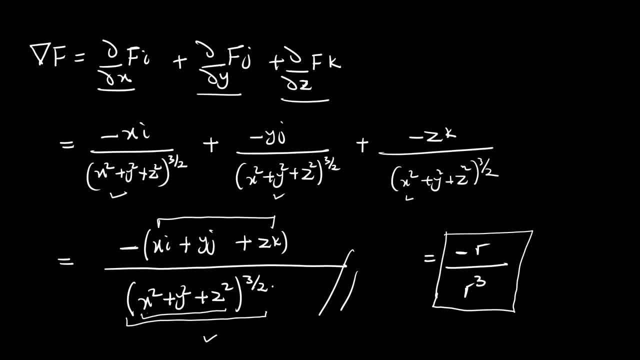 denominator, we make use of a common denominator and we add all the numerators. so by factorizing out minus, we're going to have this and this is going to be the answer to our gradient of f, which is nabla f. let's look at another example, example 2. this is a more simpler example. 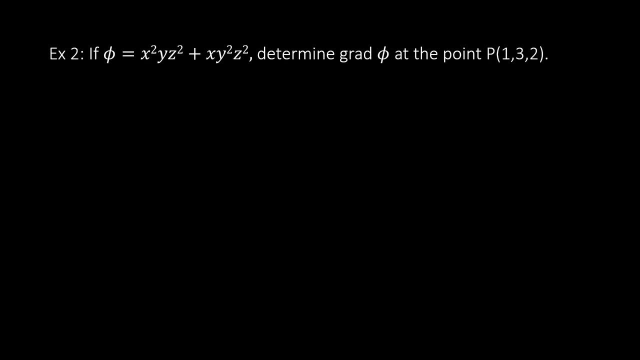 he said: if phi equal to x squared, y squared, z squared, plus x, y squared, z squared, determine the gradient of phi. at the point one comma three, comma two, we have to determine the gradient of phi and we're given a point, in this case, which is the point p, which equals to the point one comma two. 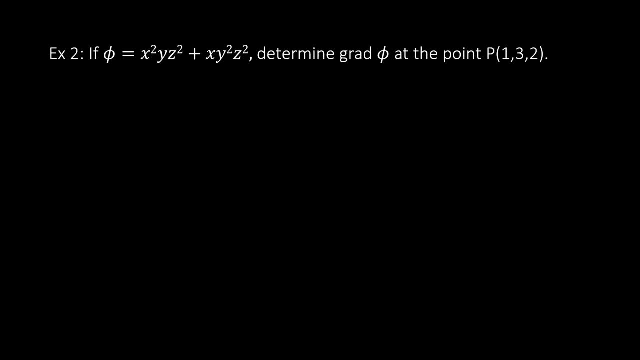 comma three. so the same thing we are supposed to do here: we look for the gradient of phi, which is nabla phi. then, after we've already gotten our answer, we substitute our point to be one, three and two. so we're going to substitute x to be one. 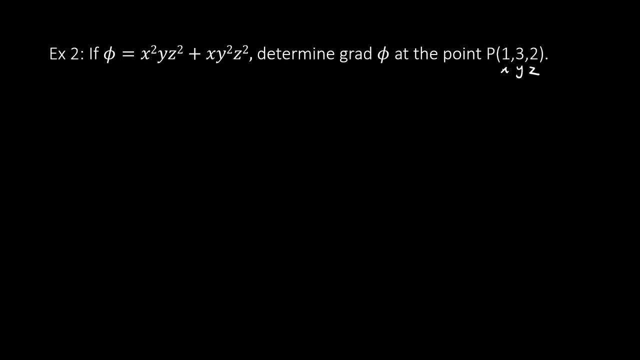 y to be three and z to be two. so let's get started with this question. so we are looking for the gradient of phi, which is nabla phi. so number five will be equal to partial derivative which will go to x of phi in direction of i. 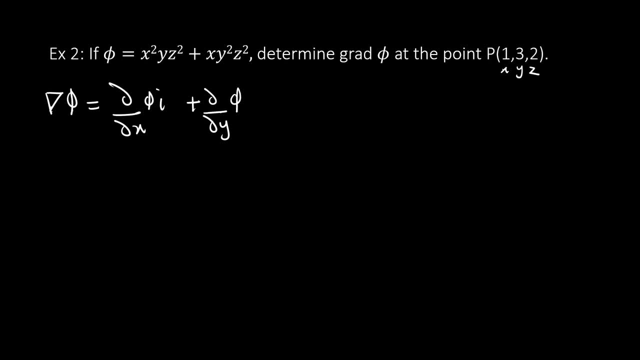 the special derivative which was made to y of phi in direction of j, plus partial derivative of phi with respect to z in direction of k. so let's do this one after the other. the first i'm going to be looking at is the partial derivative of phi. 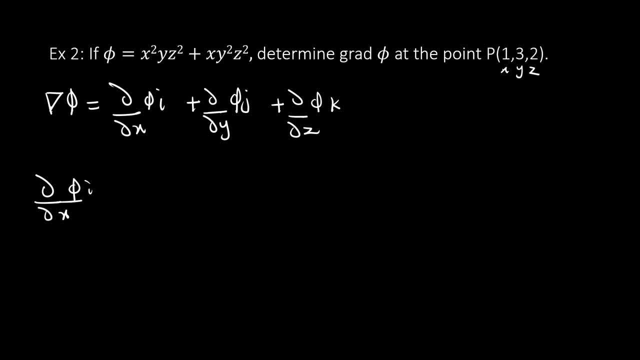 which results to x in the direction of i. so since i have my phi to be called x square, y, z squared, plus x, y squared, z squared, let's differentiate phi now with respect to x. if i differentiate with respect to x, we treat f of that term as a constant. so if we differentiate this with respect to x, we are going to have: 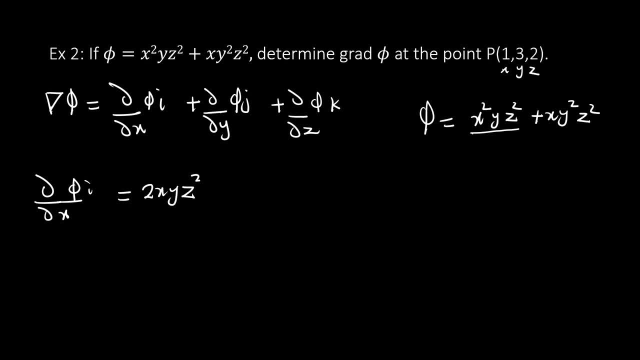 two, x, y, z, squared. now we are differentiating with respect to x and we are treating y, z as constant, plus y square, z squared, and then we're going to have i to the partial derivative of phi, which is y in direction of j. it's going to be now, if you are, 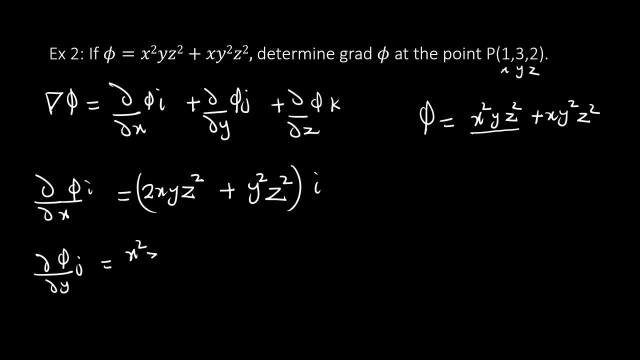 differentiating y, in this case going to be x squared, z squared plus 2 x, y, z squared and this direction of j. and finally, if you are differentiating phi with respect to z, let me put this here: if I differentiate phi with respect to z in directions of j, oh sorry, in direction of k, this is going to be: 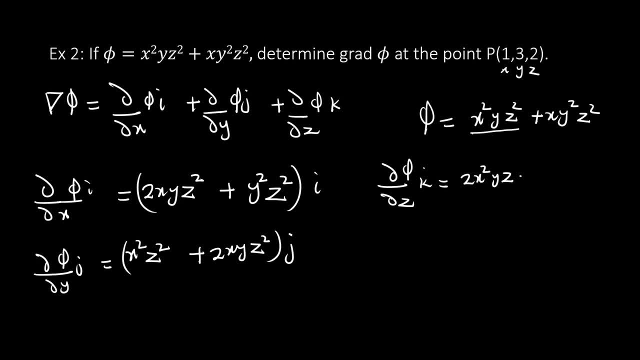 2 x squared y z plus 2 x y squared z. here we are differentiating phi with respect to z, and this is k. so we have the first term a, the second term and the third term. so bringing these three together, we are going to have 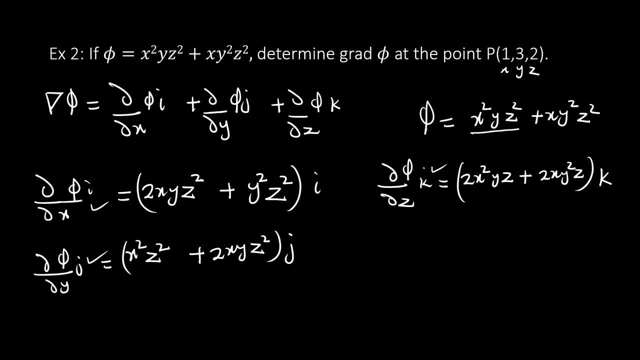 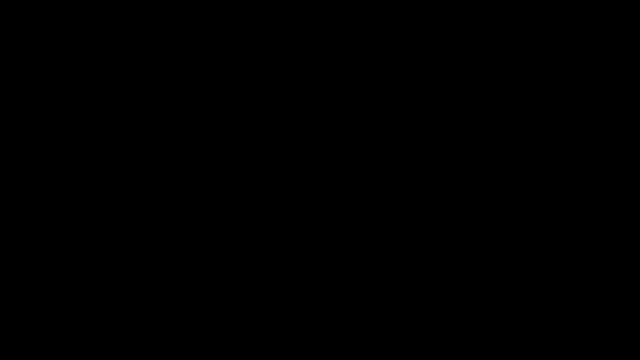 our nabla phi, which is the gradient of phi. and to wrap it up, we have nabla phi equal to 2x y z squared plus y squared z squared i plus x squared z squared plus 2 x y z squared j plus 2 x square y z plus 2 x y. 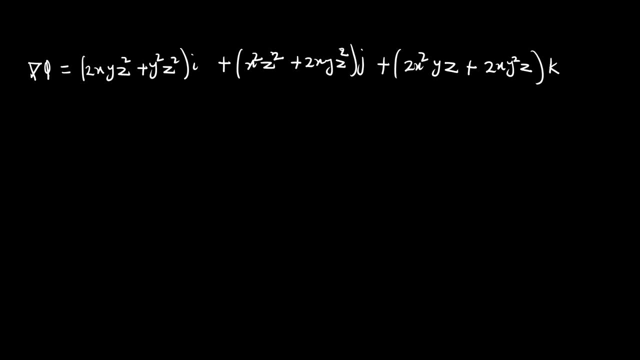 squared z. okay, so this is our nabla phi, which is the gradient of phi. but one peculiar thing in this case is that we have to find the gradient at the point p, defined as 1 comma 3 comma 2. so we simply put x to be equal to 1, y to be equal to 3 and z to be equal to 2.. so let's write our nabla phi. 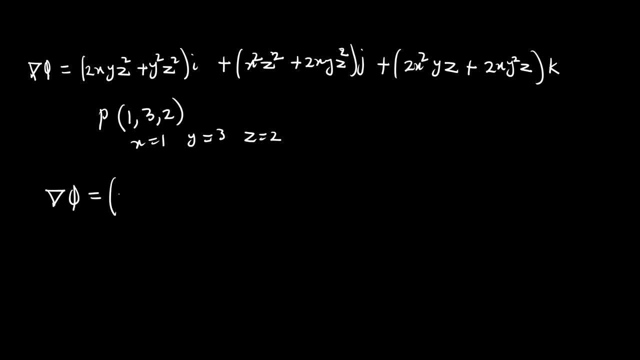 again. so nabla phi is going to be equal to 2 multiplied by x. x is 1. multiplied by y, y is 3 and z squared, that is 4 plus y. y is 3 squared, which is 9, multiplied by z square, which is 4. 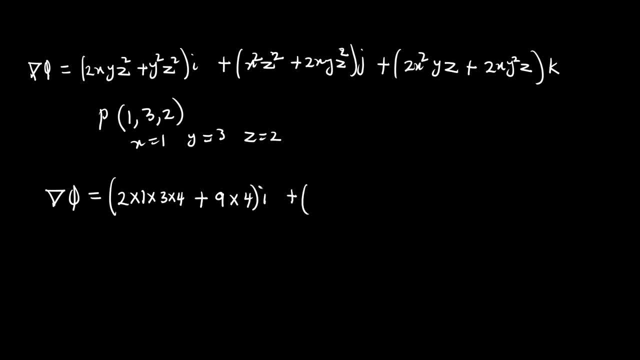 i plus the same case. here we have x square, which is 1, multiplied by z square, which is 4 plus 2, multiplied by x, which is 1, multiplied by y, which is 3, multiplied by z squared, which is 4, j plus 2, multiplied by x squared, which is 1, multiplied by y, which is 3, multiplied by z, which is 2, 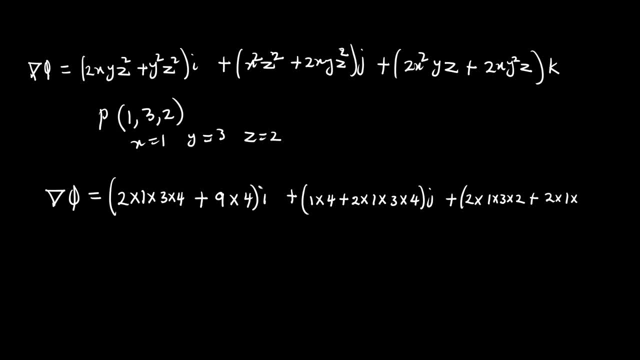 plus 2 multiplied by x, 1 multiplied by y squared, which is 9, multiplied by z, which is 2. okay, so, simplifying this, we are going to have our nabla phi. so let's simplify this together. for the first case, we have 2 multiplied by 1, that is 2, multiplied by 3, that is 6, and this is 24.. 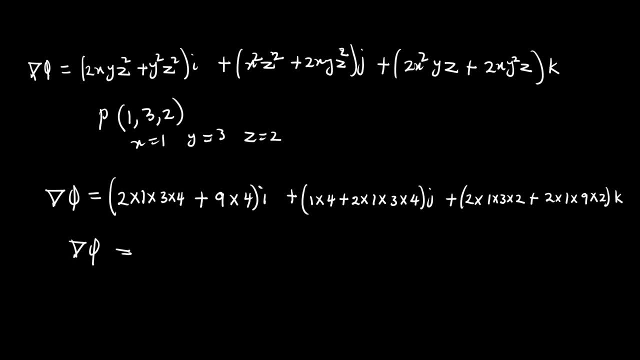 so we have 24 plus 9 times 4.. let me just write the answers. so here we have 60 i plus 28 j plus 48k. so this is the answer for our gradient, which is nabla phi 60 i plus 28 j plus 48 k. so this is that's simply how you can. 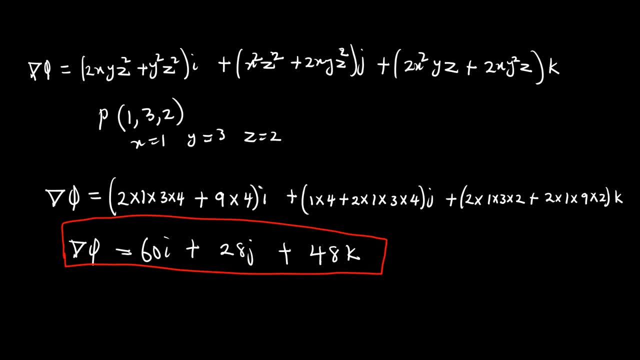 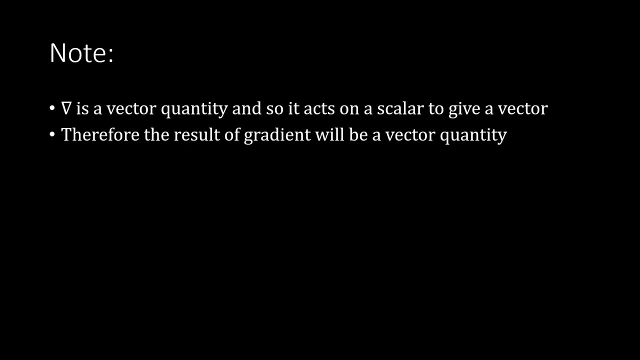 look for the gradient. if you are given a specified point, and that is that concerning gradient, try to lay your hands on one example to get this. but if you have any question, feel free to post the question in the comment section below. thank you, and lastly, before we round off this topic, i'll just 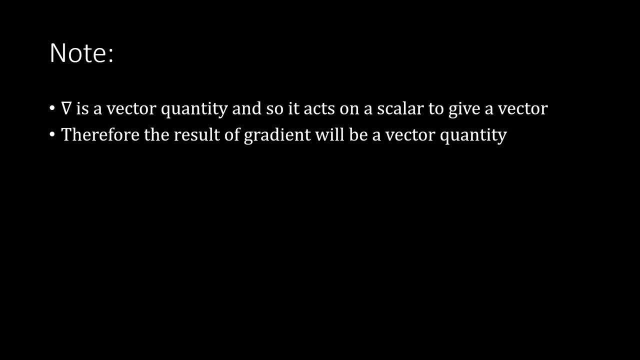 take a look at some things. so we should know that nabla is effective quantity and so it acts on a scalar to give a factor. so whenever we are talking about gradient, the function that we're going to give it's going to be a scalar quantity, as you have seen up in both of our cases, both d, f and phi. 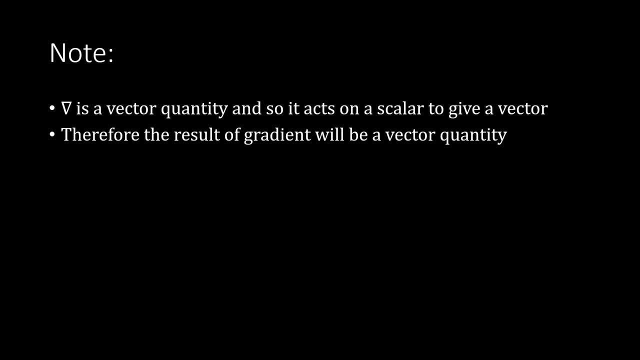 they are both scalar quantities, but nabla is in effect of quantity. therefore, the results of gradient will always be a vector quantity, as cameras. that all our answers, the only of i, j and k. so the answer is going to be in vector quantity. nabla is a vector quantity. for gradient, the function is going to be a scalar. 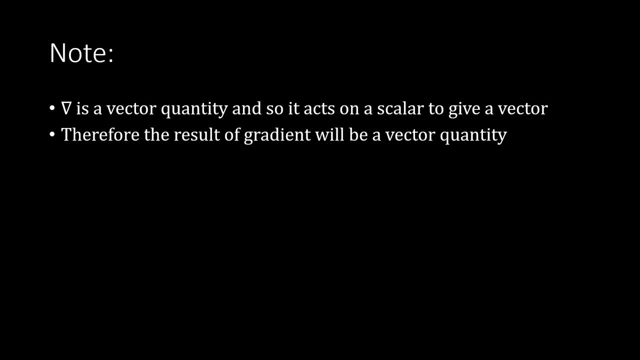 quantity and the answer is going to be a vector quantity. thank you, the second quantity we are going to be looking at is the divergence. when we look at gradients, now let's look at divergence. so let x, which is a function of x, y, z, equal to x 1, i plus x 2, j plus x 3, k, be a differentiable. 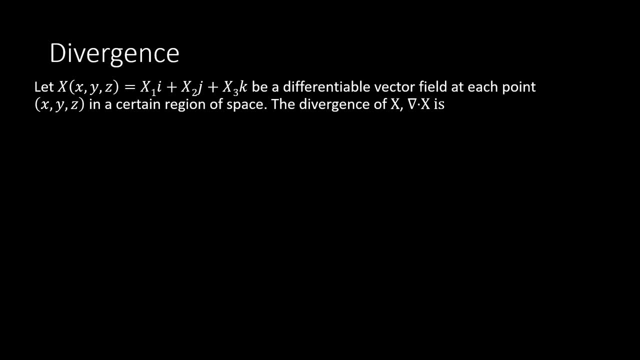 vector field at each point- x, y, z- in a certain region of space, the divergence of x, which is defined as nabla dot x. now i want us to take the notes of something here: when we are looking at gradient, we say that gradient is represented as nabla x or nabla f, which is f is our function. 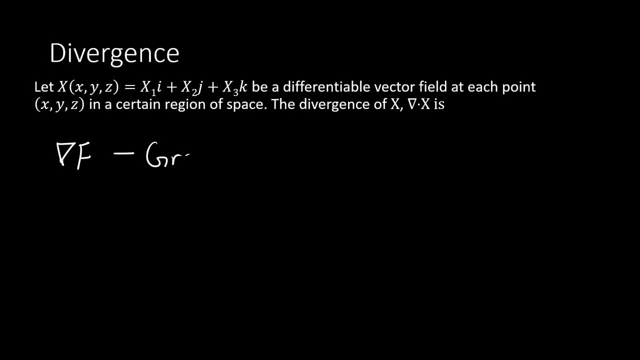 so in this case we say that divergence this is gradient and this is divergence. nabla, dot f, this is divergence. so what we should take now is that divergence will be treated like a dot product of vector. in case of gradient, our function is solely in scalar quantity. but in this case our function 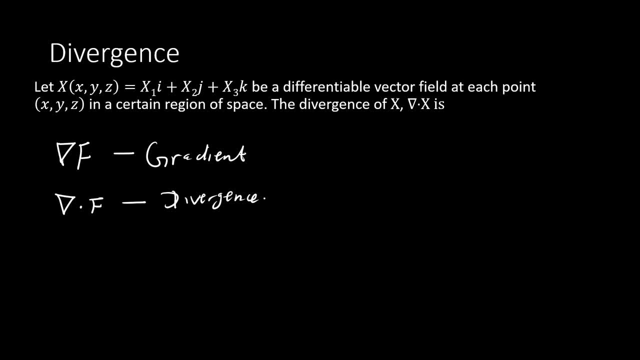 is going to be a vector quantity and since we know that our nabla is a vector quantity, then we are going to treat the two like a cross, a dot product. so we're going to take the dot product of nabla and our function f to get our divergence. so let's look at how we can represent our divergence. let me let me clean. 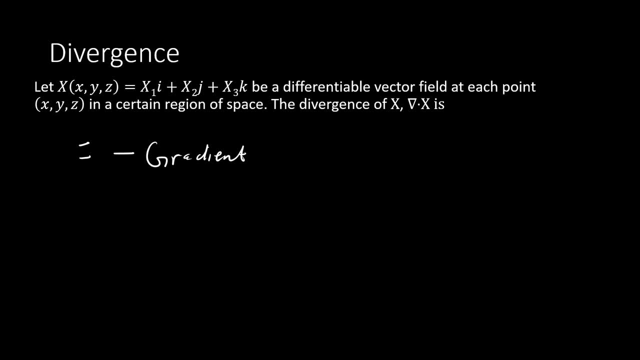 this off, as i mentioned that we're going to be using nabla. very well, so our nabla dot x is defined as i plus partial derivative with respect to y, j plus partial derivative with respect to z. okay, dot products: x1, i plus x2, j plus x3. okay, so this is how our divergence will be represented. 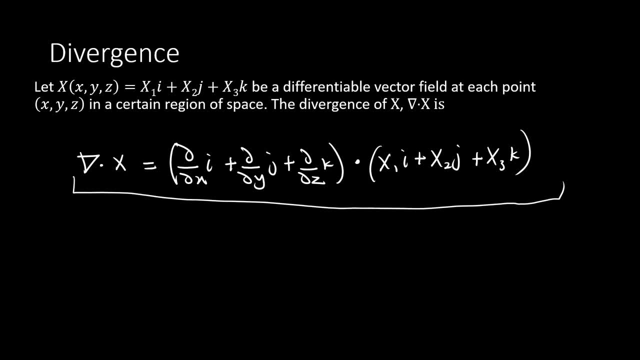 the product of nabla and, and z and x the dot product of nabla and x. so let me just do a quick reminder for us concerning dot products. now we should know that if you are multiplying two vectors, if you are taking the dot product of two vectors, we are going to have a scalars. our answer let's. 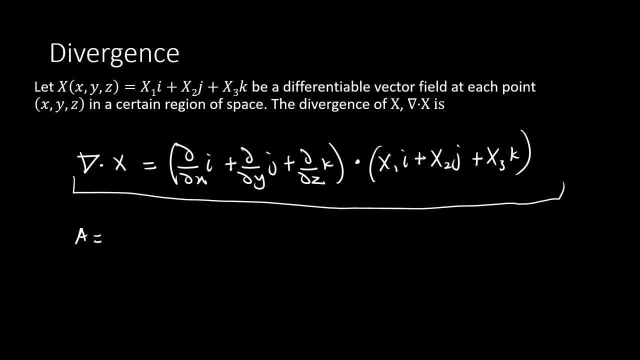 look at just a quick example: if you have a to be equal to 2 i plus 3, j plus 4k and we have b to be equal to 5, i plus 3 plus 6, j plus 7k and you have to look for a dot b. 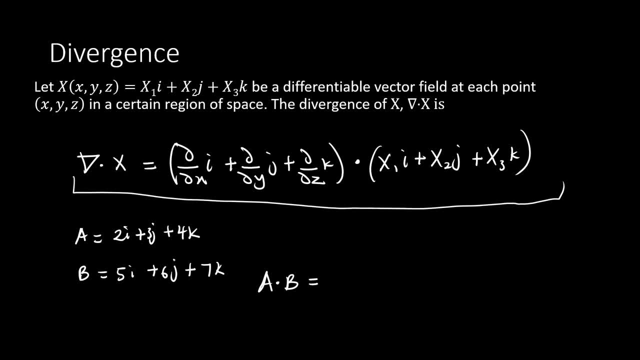 which is the dot product of a and b. so what's happening is the quantity i is going to multiply like each other: the j will go for each other and the k will go for each other. so you're going to have 2 times 5, which is 10.. if i multiply by i, we are going to have 1, so we are not going to write. 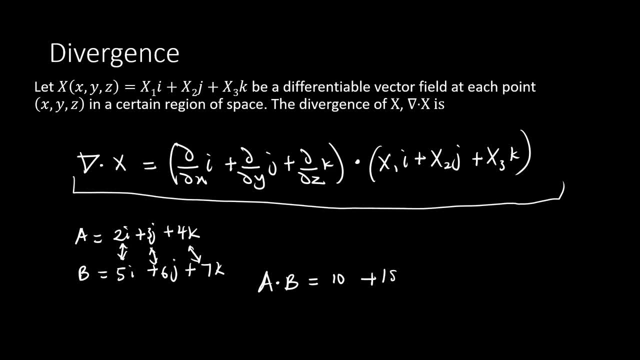 that again plus 3 times 6, which is 18, plus 7 times 4, which is 24, sorry, 28. so this is how dot product goes. then we add this: this is 28, 28 plus 20, that's going to be 56.. so this is how we do dot product. 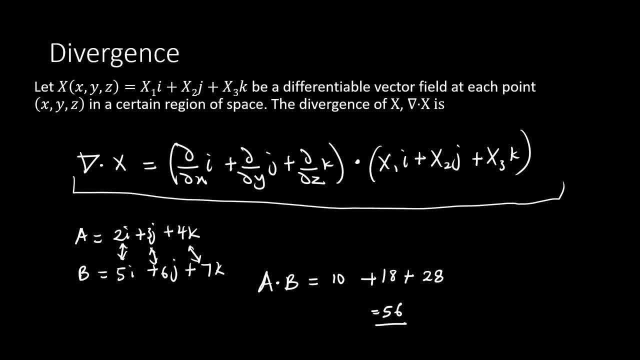 the same thing is going to be applied in the case of divergence there. if you have two vectors, which is nabla, and our function, which is defined as b, maybe in this case. so we're going to have our dot product of a and b, which is the dot product of nabla, and our function to be equal to a dot b. 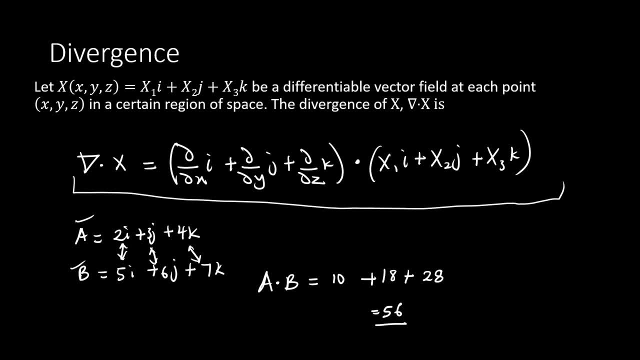 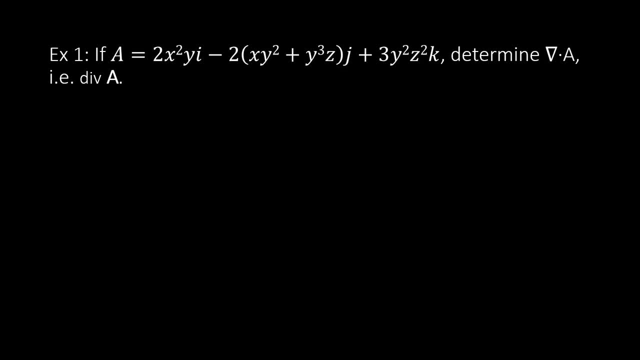 and this is i will go for i, j will go for j and k will go for k. let's start by looking at some examples. so, except one says: if a equal to two x square y, i minus two, into brackets x, that is the divergence of a and that is nabla dot a. so we are looking for nabla dot a if you. 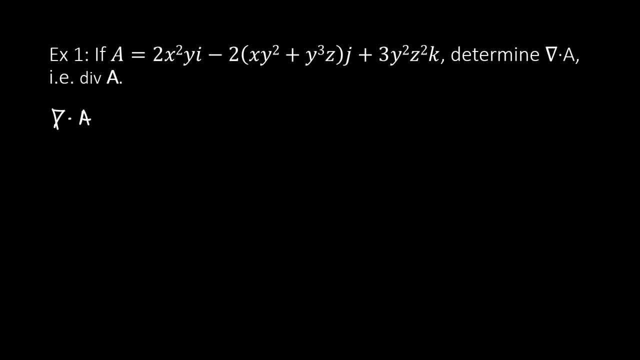 are representing divergence. don't forget to put this dot. that's what differentiates between divergence, call and gradient. so divergence is nabla dot a. so, as i mentioned before, we have- okay, let's write this- so we have our nabla to be equal to xi. we take note of this from the beginning, that this is how we represent our nabla. 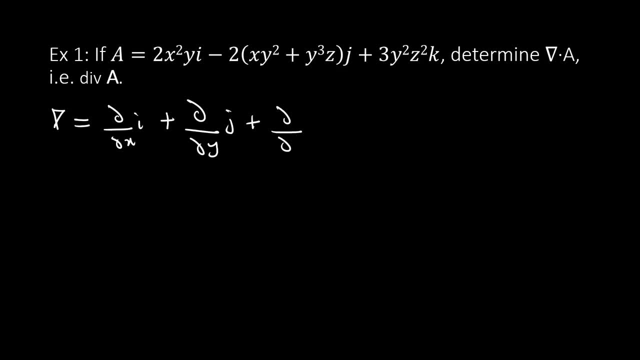 this is j plus and this is k. and also we have a to be equal to 2x square y i plus 2 to bracket x y square plus y cube z j plus 3 y square z square. okay, so we are looking for nabla dot a. so 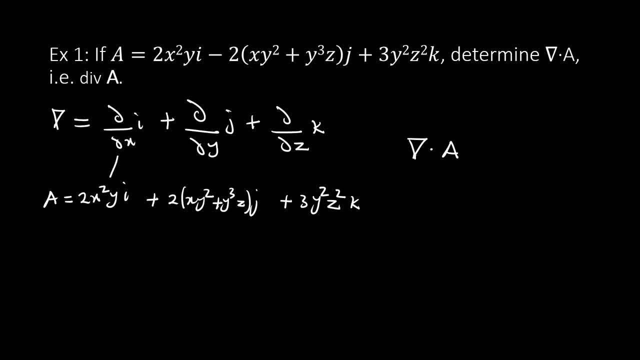 this is dot product. this will go for this, this will go for this and this will go for this. so let's start by looking at the first one, which is partial derivative, which is respect to x of two x square y. so it's like you're multiplying this value. by my idea again. so we simply write out this by this, this one, this multiply by this. if you multiply i and i, you are going to have one. so you owre going to negative 1 other than this. you are going to put the proof by i addi i again. so you simply write out what is equal to one times i. so you simply write out what is not equal toВ 2x2 y. so you multiply by this. this will do it. 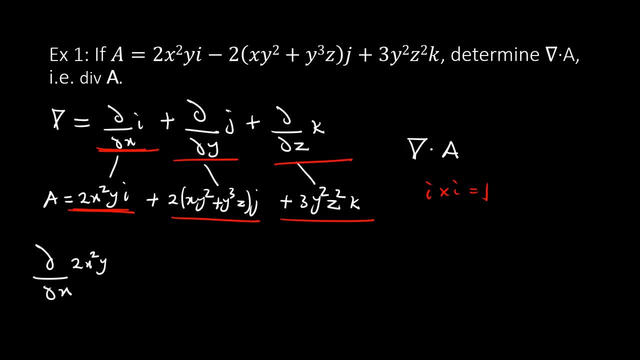 which is d over dx to x square y. so if you have to differentiate this with respect to x, this is going to go to 2 x. no, this is going to be 4 x- y. if you get that here, you're going to have partial derivative which is equal to x. 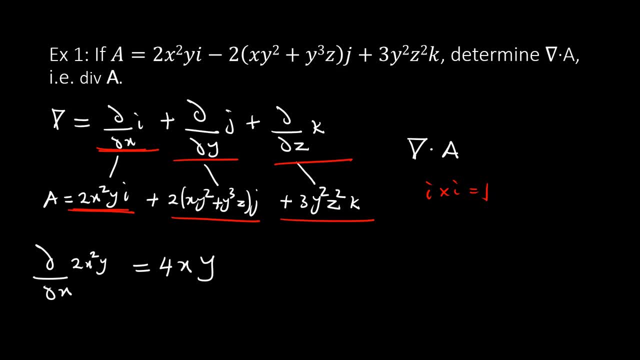 of 2x square y, to be equal to 4 x y, and the second, which is, which is equal to y of 2, let me, let me multiply it through this bracket and we are going to have 2 x y square. i sorry, this is g. 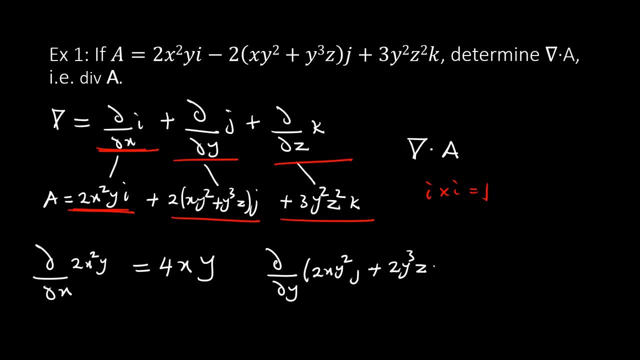 plus 2 y cube z g, so that what i did is just to multiply, just open the brackets, so i must fly through by y cube z g, so that what i did is just to multiply, just open the brackets, so i must fly through by two. and 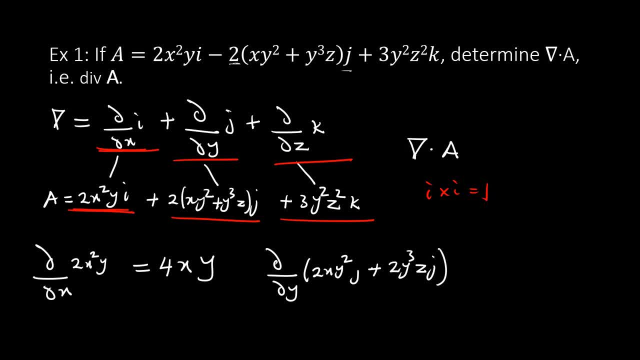 also by j. so if to open these brackets we have two x, y square and also j is going to be attached. plus, if 2 comes to this place also, we have to y key z and also j will be attached. so let's differentiate this with respect to. 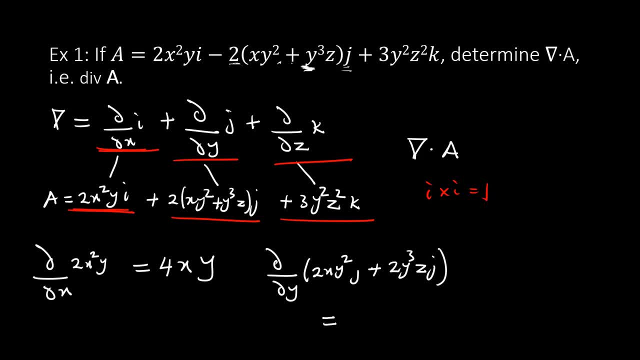 y, and this is going to be 4 x y j plus six y square z j. it's very necessary. we put the bracket there because of this negative sign. so if you differentiate this with respect to y, we are going to have four x y j plus six y square z j. so now let's do the third one. 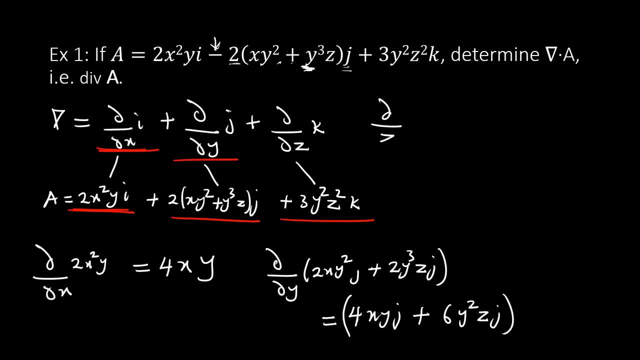 so now we have to differentiate, with respect to z, of three y square z square, and this is going to be six y square z. now I'm differentiating with respect to z: this is going to be six y square z. so now we have our first value, this. 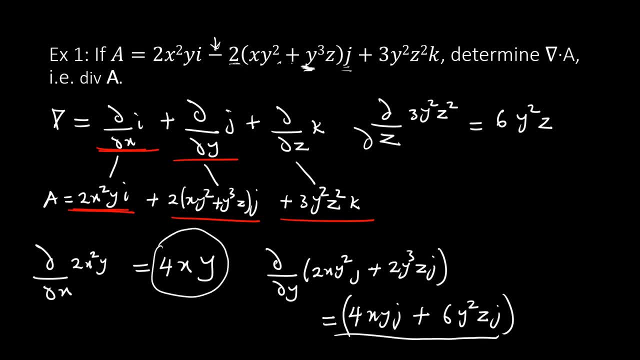 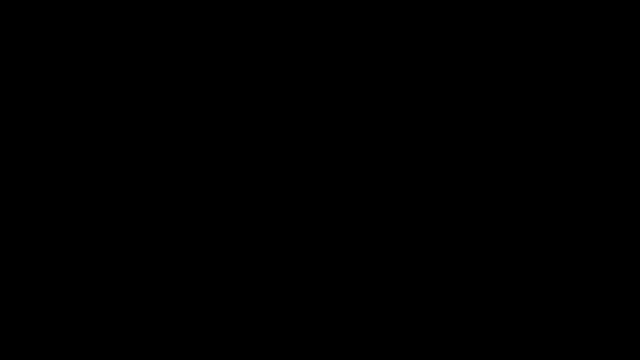 is what we have first. we have this and we also have this. so just joining these three together, we have our divergence of a, which is div a. so let me write the answer on another page. so we have diff a, which is the divergence of a, to be equal to. 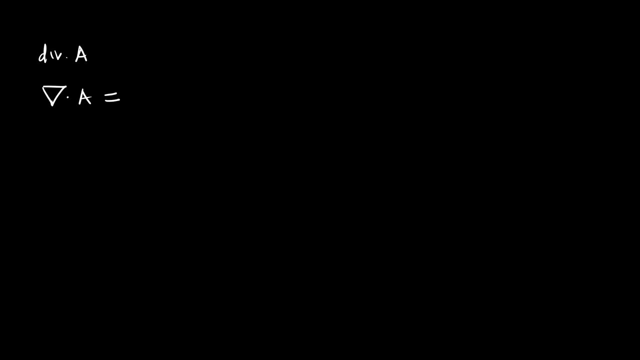 4 X Y minus 4 X Y G plus 6 Y square Z, J plus 6 Y square Z. oh, sorry for this. j is not going to be attached again. sorry for that. our answer is supposed to be a scalar constant, so j is not going to be attached again. sorry for that. 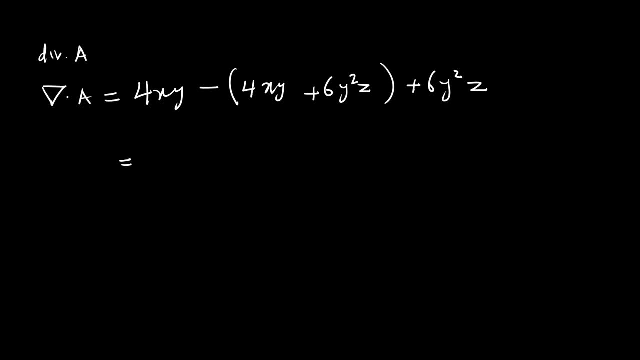 so we have? the answer is to be: if you open the bracket through, we have X Y minus 4, X Y minus 6 Y square Z plus 6 Y square Z. so this will cancel out. this will cancel out. so now, this is interesting- we now have: 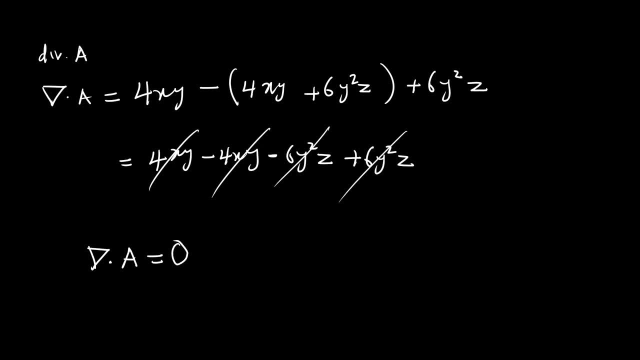 the definition of A to be equal to 0. Wow, so we have the definition of A to be equal to 0. I hope you get that. so you have the definition of A to be equal to 0. so why is the definition of A equal to 0? 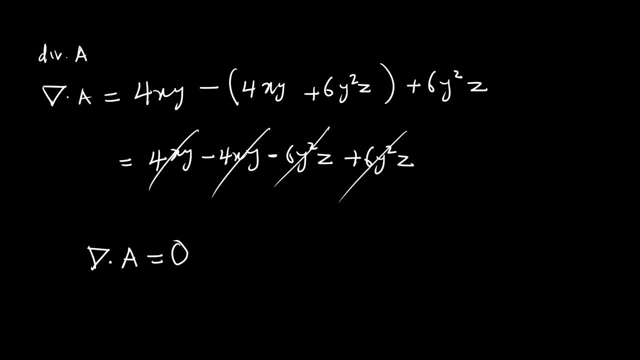 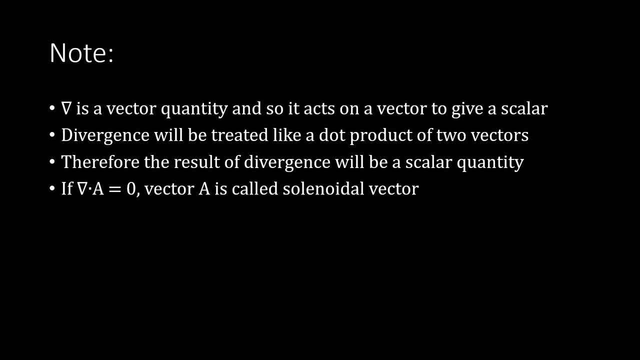 there's something you have to take notes, so let's take note of some things. so what if you have definition to be equal to 0? what does it mean? so let's look at some notes. so you should know that nabla is a vector quantity, and so 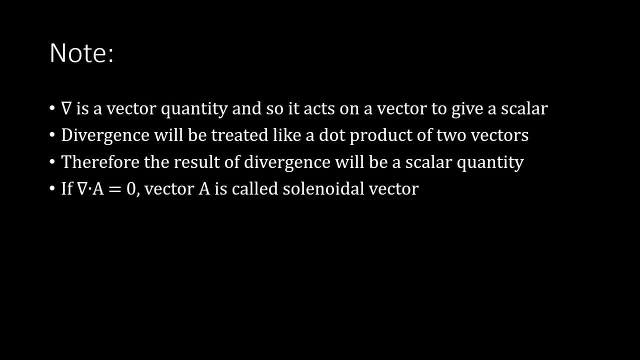 it acts on a vector to give a scalar. this is the first thing we are supposed to note: that nabla is a vector quantity and also our function that we're going to be given is going to be a vector quantity. so when there's a dot clause between the 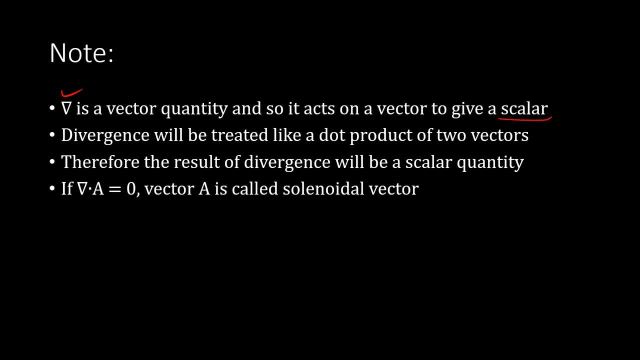 two vectors, we're going to get a scalar quantity, and second one is a divergence- will be treated like a dot product of two vectors. after i talk about that, divergence will be treated like the dot product of two vectors. so therefore, the result of divergence will be a scalar quantity and whenever we have divergence equal to zero- this is the fourth. 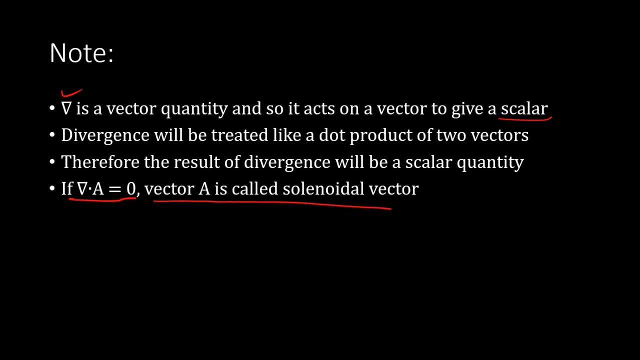 condition, the vector is called a solenoid vector, just like what we have in the previous example. so the previous example is a solenoid vector. so whenever divergence equal to zero, the vector is called a solenoid vector. thank you, let's talk about call, call. this is the last quantity we'll. 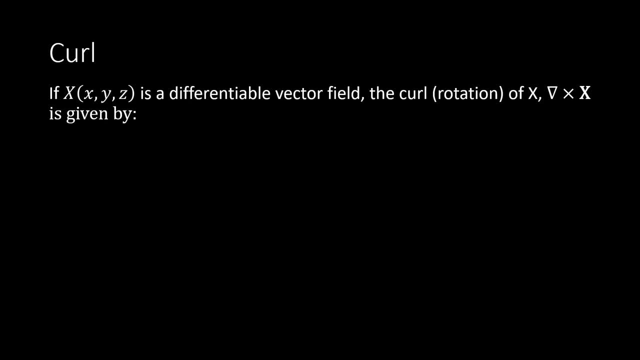 be looking at call. so if x, which is a function of x, y, z is a differentiable effect of it, the call which refers to us the rotation of x, is given as nabla multiplied by x, nabla multiplied by x. and now this where we have to take note of another function. 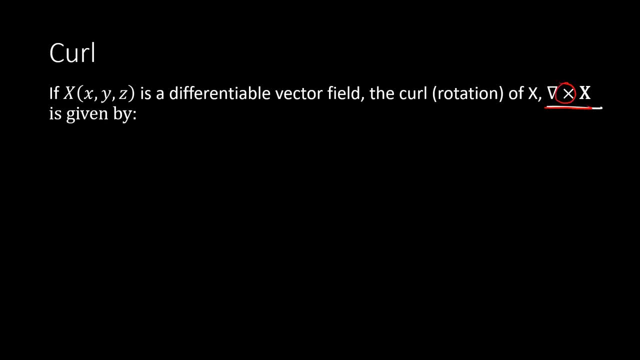 you, which is the cross product, for the case of divergence is going to be a dot product, but for the case of call is going to be a cross product. that's what you just have to take note. but the case of divergence is a dot product and therefore the case of call is going to be a call, a cross product. so let's see how we can. 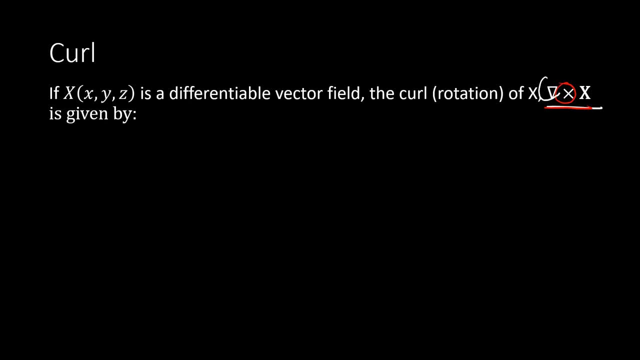 represent our call, the same way we have been representing. nabla is nabla. you just have to find the way of representing x. so nabla multiplied by x is going to be so our nabla is. but i try to fit it with respect to z, k. so multiply by however we are defined, however, 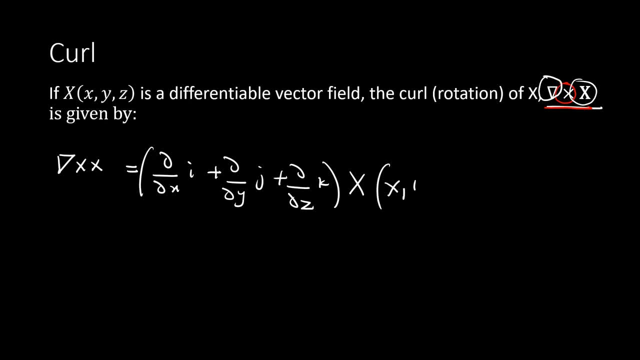 they define our x. let's find that x1 i plus x2 j plus x3 k, and this is going to be the factor product of two vectors. so how do we represent this? let me clean this off. i hope we get that. so let me clean this off and let me represent it how we represent, how i will represent. 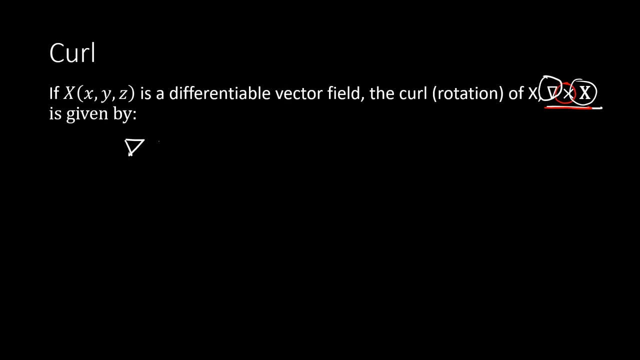 a cross product. so nabla multiply by x is going to be given like this. if you recall this, when we look at our factors, this is how we are going to be representing cross product. this is i, j and k. this is relative with respect to x, reset to y and respect to z. 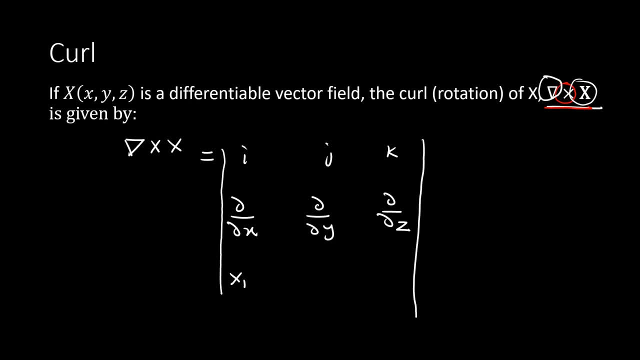 and this is going to be x1, x2 and x3: x1, x2 and x3. so this i will represent our call. this is a vector product of two vectors, which is vector nabla and our vector valued function. so let's to get this very well, let's. 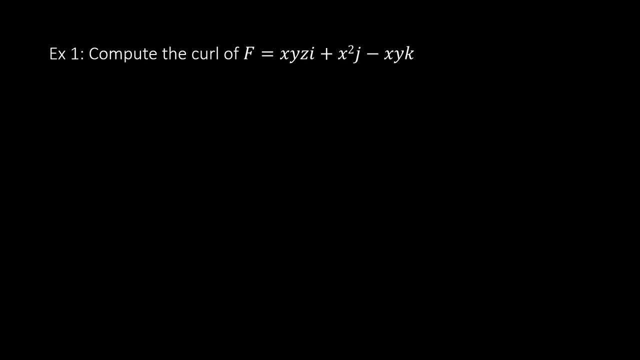 look at some examples. these are: affects the sample compute, the call of f equal to x, y, z, i plus x, j plus x, y minus x, y, k- we just go straight to the answer here. so we have to be equal to this: i, j and k. it's a partial derivative of x, a derivative which relate to y. 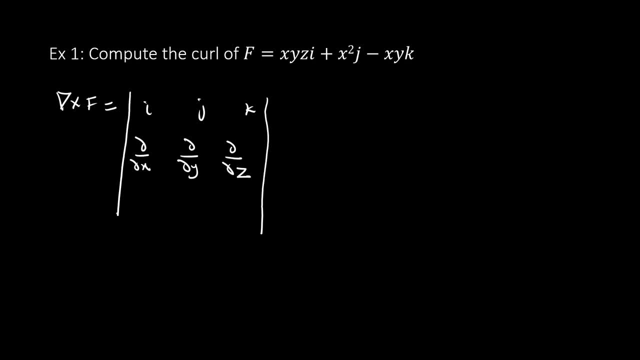 we have derivative with respect to z. i'm going to write out our function one after the other. this is x, x, y, z, this is x square and this is minus x, y. so you can see that for i, i put this, for the case of j, i put this and for the case of k, i put this. so this is going to be arranged just like if you are. 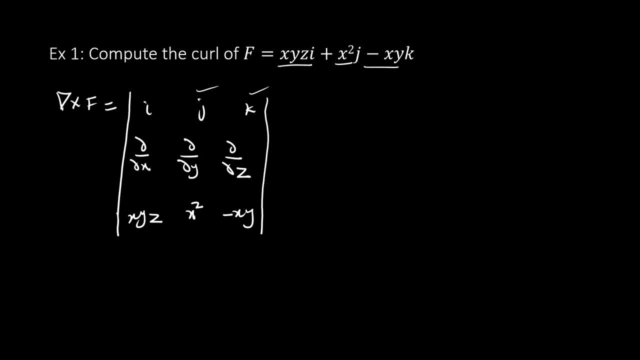 doing a cross product of two vectors. now let's solve this. so this is going to be solved exactly the way we solve the cross product. first let's look at: let's cover a 1- 1 if you cover this up. so we are going to have the first one to be equal to. 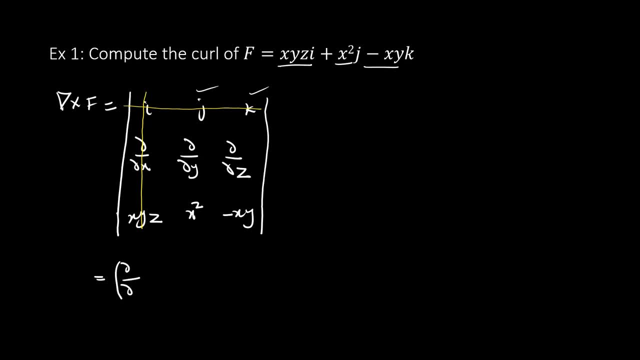 this: this is plus and minus, so this is going to multiply this and this will multiply this. so it's minus x y, so minus derivative with respect to z x square. so that is for a 1 1, for a 1: 2, we cover this and this. 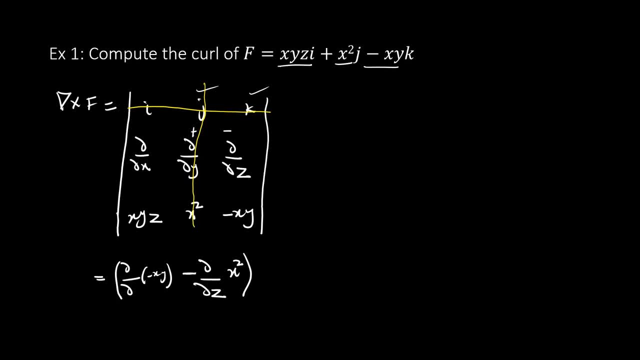 so what we are and this we are going to forget, we are going to have add i a, so now we are going to add. so i will say: first one, to be honest. i like to give you another example one more time. this is one. and last one, to be honest, this is i don't know, but i have given it two. 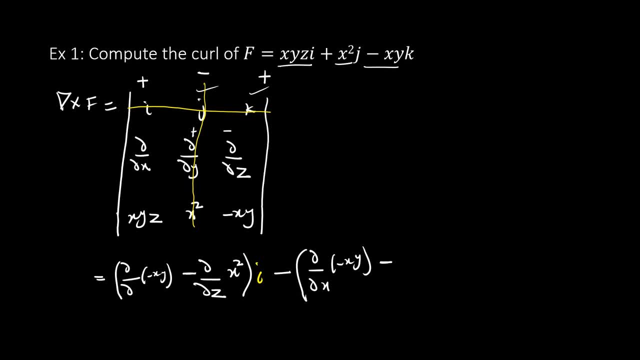 instead of one, so this one. to be honest, if we take this plus and let me show you, let me show you, let me show you this side as well, the device that we are estranging, this is plus and plus. we have minus, we have minus, this is going to have j plus. so we look at this this much like this: 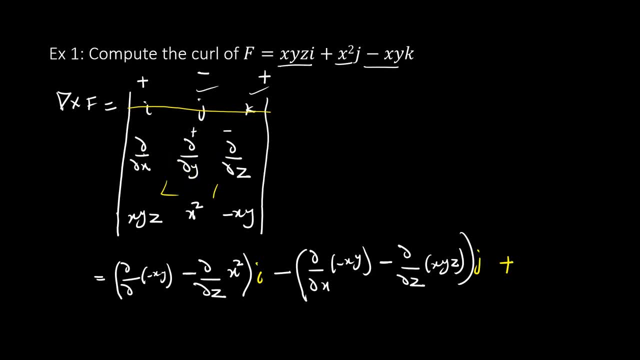 let's try this for this case. so let's look at a, one, three, so we are covering this and this. so you have plus. let me put this a, let me put our key. so if you simplify this now, that's going to be our answer. so simplifying this will exactly be our answer. 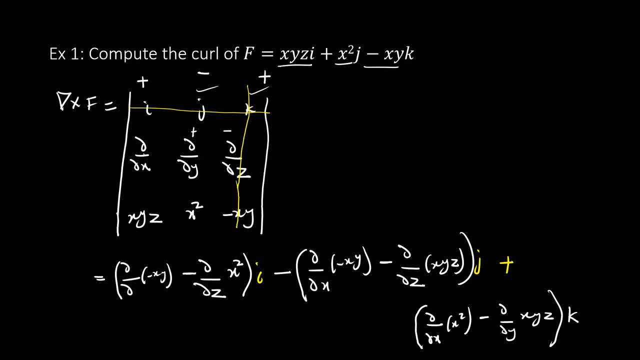 so let's try, if we can still write the answer on the same page. so i'm going to be putting down the answer. so, if i, if you differentiate, this is: oh, what's going to be there. this is the y. sorry for that. so if you differentiate this with respect to y, we're going to have 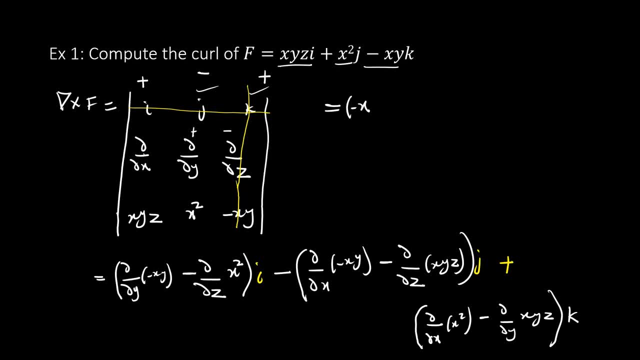 minus x. and if you differentiate with respect to z, since there's no z here, it's going to be like the differentiative derivative of a constant, and that is zero plus zero is i plus. so if you had this minus, sorry, so differentiated this with respect to x. this is going to be minus y. 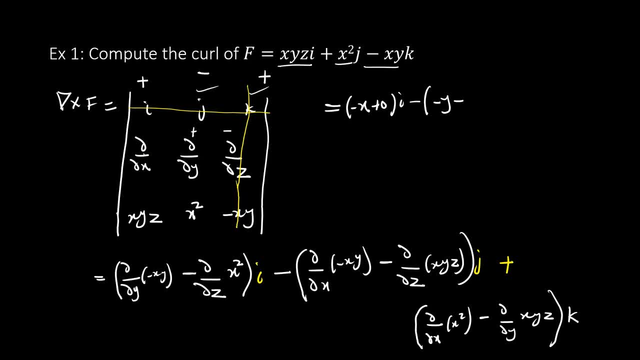 minus. differentiated this with respect to z, this is going to be x, y, this is j plus. so differentiating this with respect to x is going to be 2x minus, and differentiated this with respect to i, this is going to be x, z. okay, so simplifying this, for that we have. 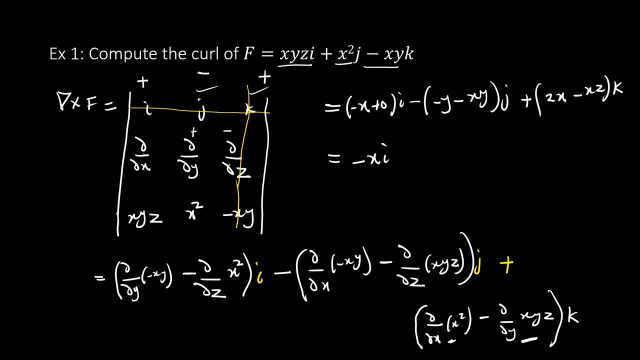 minus x, i minus minus y, minus x, y, j plus 2x minus x, z. okay, so to write that one body, we can say the answer is now minus x, i plus 2x minus xz. if we multiply 2 by minus, we have plus y plus x- y. 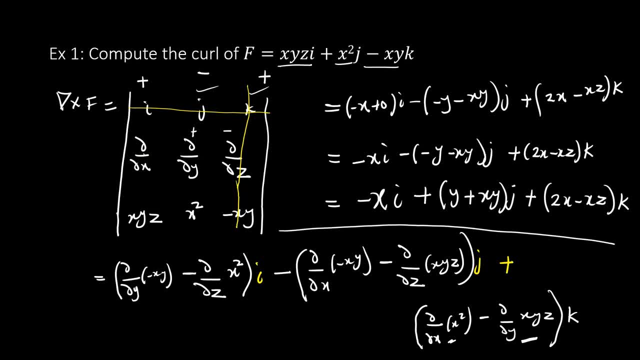 j plus 2 x minus x z. okay, and that's going to be our answer for the first example: minus x, i plus y plus y plus x, y, j plus 2x minus x z, a vector quantity, unlike the case of divergence that we have our answer to be scalar quantity. 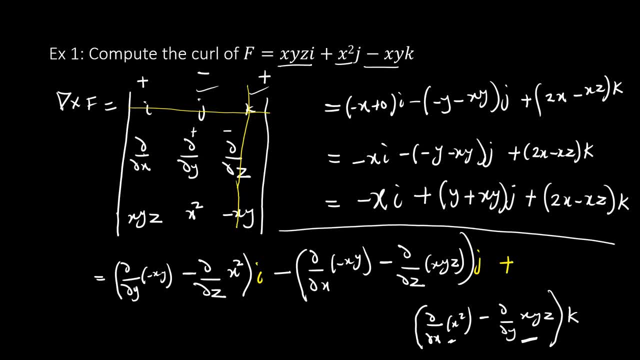 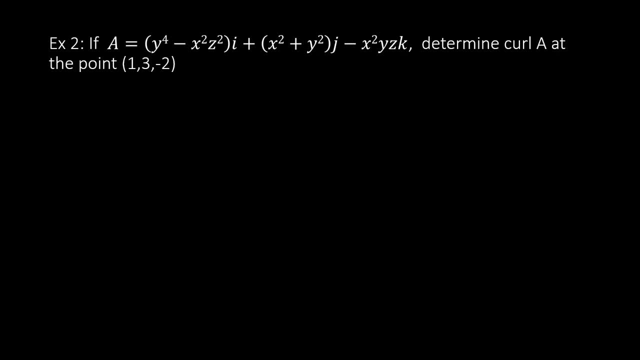 now let's look at the last example on the call. so looking at our last example, we have example two. if a equal to y to the power of four minus x square z square i plus x square plus y square j minus x square y z, k, determine the call a at: 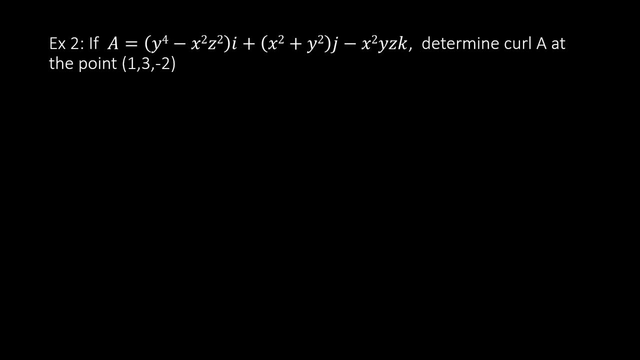 the point one comma three, comma minus two. so we are looking for the call at the point one comma three comma minus two. so, yes, we are going to go straight to our representation. so we have the call of a to be nabla played by a to be called to drawing a matrix. we have our i, j and k. 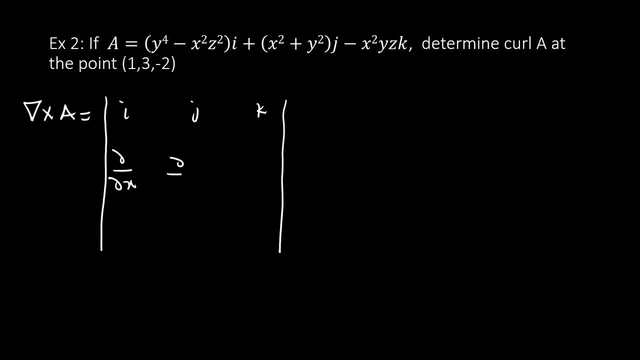 and this is by the derivative with respect to x, by the derivative with respect to y and partial derivative with respect to z. so the first file we have there is y to the power of 4 minus x square, z square, followed by x square plus y square and lastly, we have minus x square. 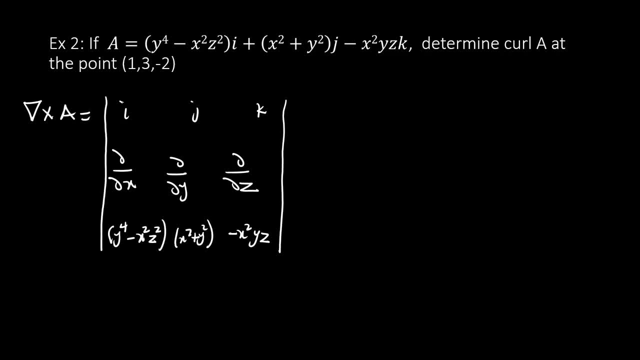 y, is it? so? to make this easy for us, we are going to be looking one after the other, we're going to begin one after the other to make this easy for us. so this is plus, minus, plus, we are canceling out our a11. so this is plus, this minus, in this case, to this much like this and this much like this. so 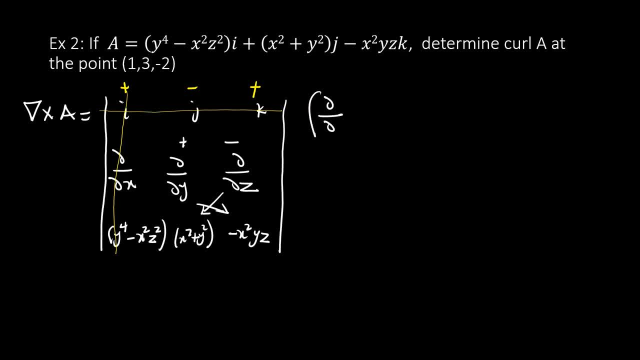 we are going to have partial derivative with respect to y of minus x square, y, z minus, partial derivative with respect to z of x square plus y square, and this we have, i. so let's try to solve this before we continue looking at the others. let's try to solve this. 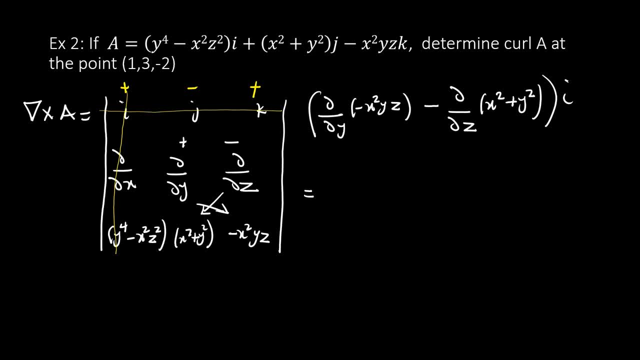 so this is going to be- or let's look at everything at the same, the same time, before you continue. so this is the first our i variable. let's look at the one for j. so if you cover out a12, we're going to have a12. 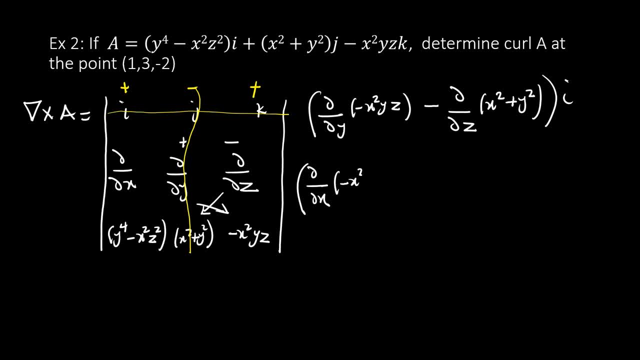 a12, a13, so jv variable and lastly, variable. so we are canceling out a13, canceling out a13, and this is going to be partial derivative with respect to x of x squared plus y squared minus. partial derivative with respect to y of y to the power of 4 minus x squared z squared. 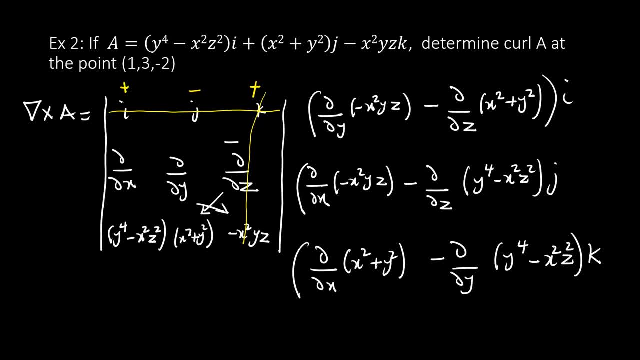 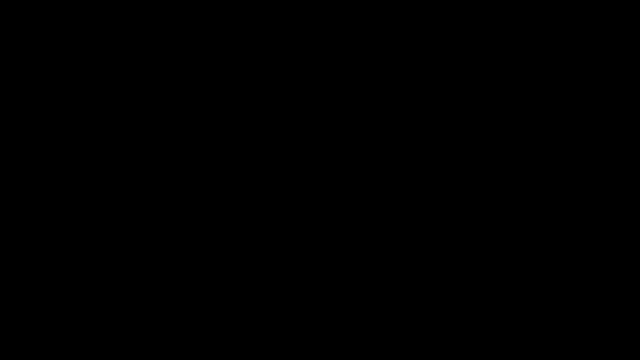 and this is our k variable. so you have our x, y and z. so, simplifying these three, you are going to have our answer. so for our i variable, we have the partial derivative of minus x squared y, z minus partial derivative with respect to z, of x squared plus y squared i. so let's find this partial derivative of this with respect to y. 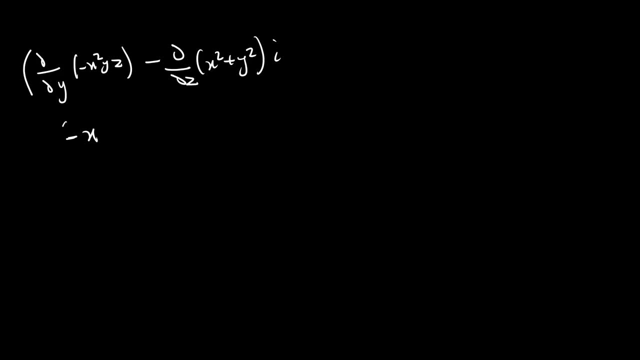 is going to be minus x, squared z, minus a supplier derivative Now, Since there's no n z here, So we can just count to the result. and this is i. so this our i variable. we are done with that. for our x, for our j variable, you have the partial derivative. with respect to x of minus x squared y squared y squared x squared y squared y squared y squared, and 2x squared x. 2 and 2x squared Из is left, z is also 0, and there's nothing other than any 그다음에, and this is i. 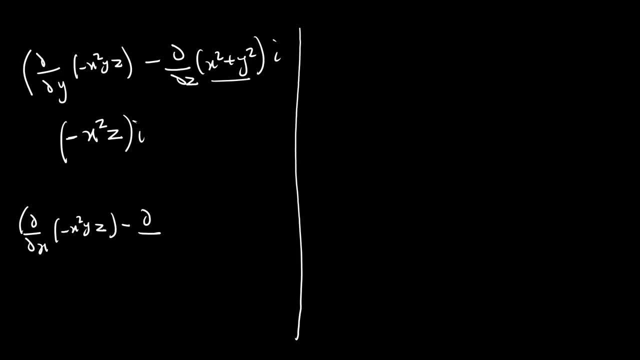 y z minus the partial derivative, which is z of y to the power of 4, minus x square z square g. so if you differentiate this with respect to x, we are going to have minus 2 x y z, and if you differentiate this with respect to z, we are going to have 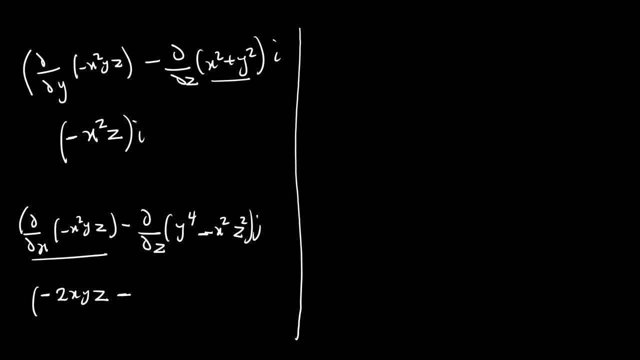 what is this minus? we're going to have minus 2 x square z. if you differentiate y, it's going to be zero, since it's not z and we are differentiating it from z. so it's only in this case that we have z and it's going to be minus 2 x square z, and this is j. so later this is going to come out. 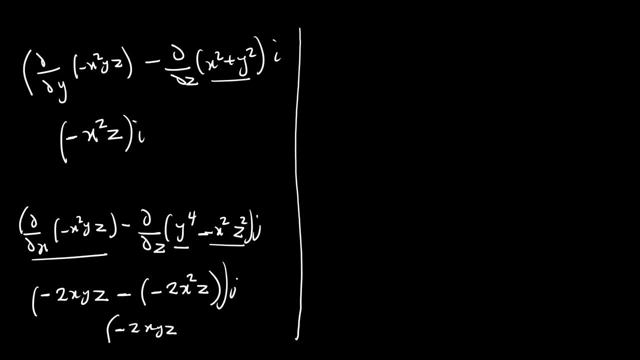 so to have minus 2 x y z. so this is going to come out. so to have minus 2 x y z, and this is going to be minus 2 x y z, plus 2 x square z- j. so that's our j variable and, lastly, our k variable. so what we are doing is: 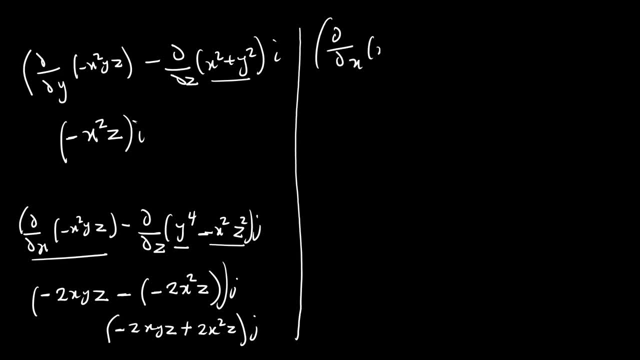 we are differentiating with respect to x of x square plus y square minus, differentiating with respect to y of y, to the power of 4 minus x square z square k. so if you differentiate this with respect to x, we are going to have 2 x. 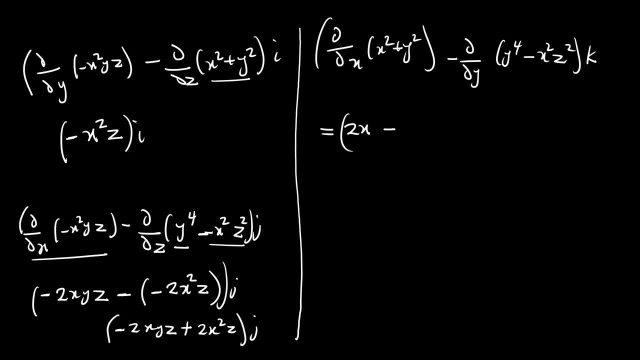 minus. differentiating this with respect to y, we are going to have minus 4 y cube and this is k. minus 4 y cube and this is k. so now we have our x y i variable, we have our j variable and now have our k variable. so what we have to do now is substitute our follow of p, which is at the point. 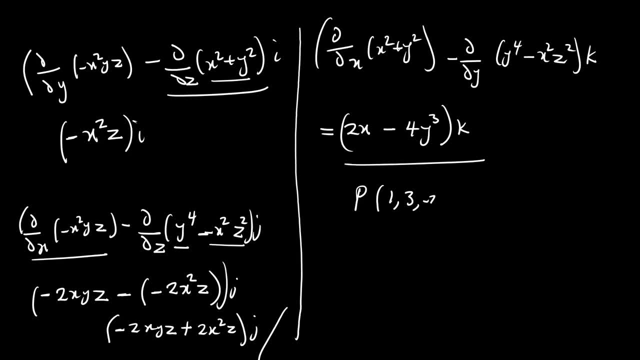 1 comma, 3 comma minus 2. so i'll just write this out, i'll punch the calculator and i'm going to write the final answers out. so the call of f, which is represented as this, is going to be equal to: so this is after you substitute the follow of x and z. there you're going to have two i. 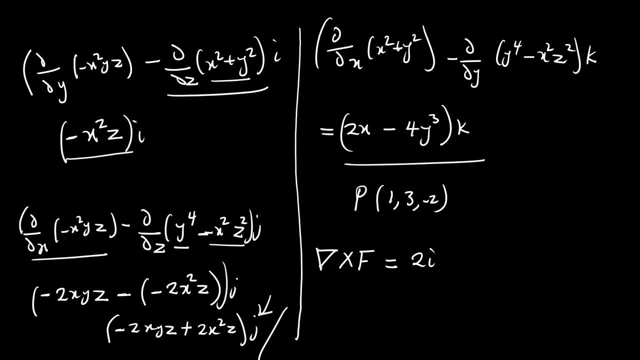 after you substitute the follow of x, y and z, j, you're going to have plus 8 j. and now substitute the follow of x and y, we're going to have minus 106 k. so this is going to be our answer for the call of f 2 i. 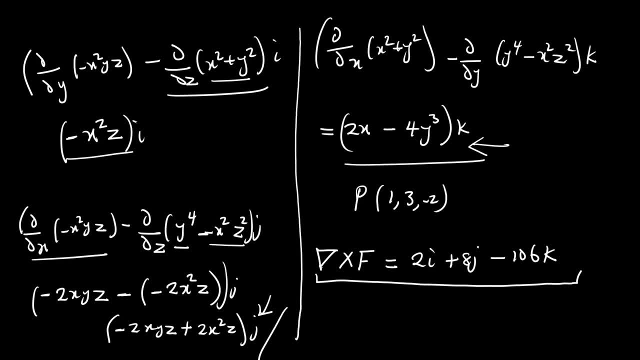 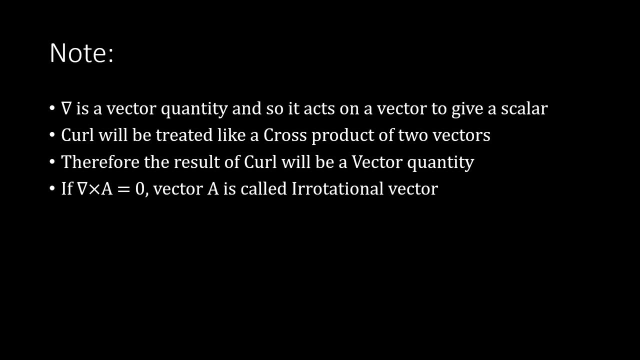 plus 8j minus 106 k, 2i plus 8j minus 106 k. and that is that if you are asked to find the call at a particular point, and to cap it all, let's take note of this note also. we know that 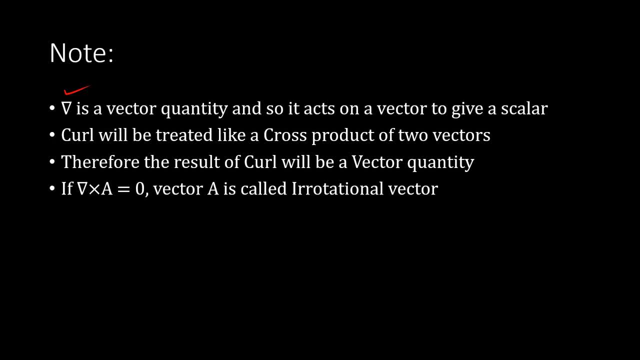 our line is a vector quantity and it will act on the vector quantity to give a scalar. so call will be treated like a cross product of two vectors. as we mentioned before, call is going to be treated like a cross product of two vectors so therefore the result of call will always be a 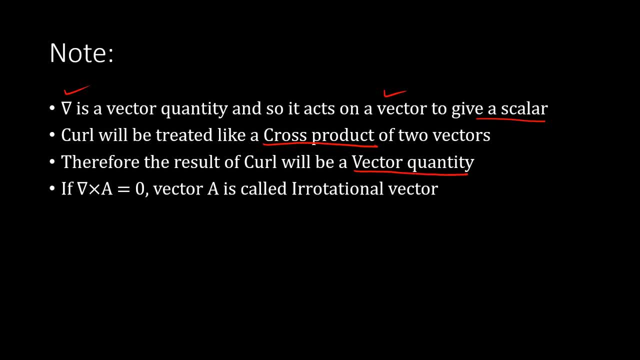 vector quantity. the result of call will always be a vector quantity and if you have your call to be equal to zero, if the call is equal to zero, the vector is referred to as irrotational vector. so, and that is that concerning call. so, to round off this tutorial, i want you to try this if phi.